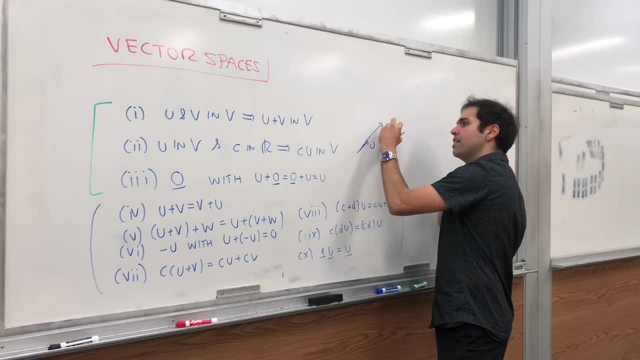 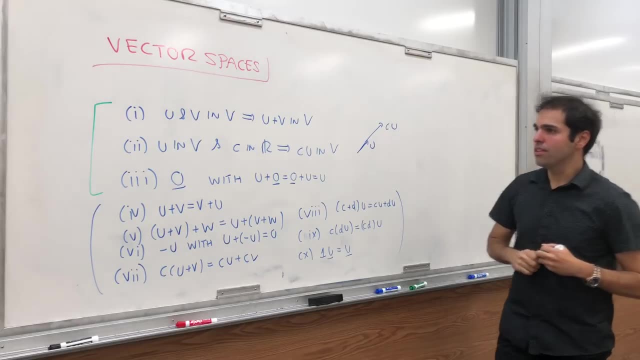 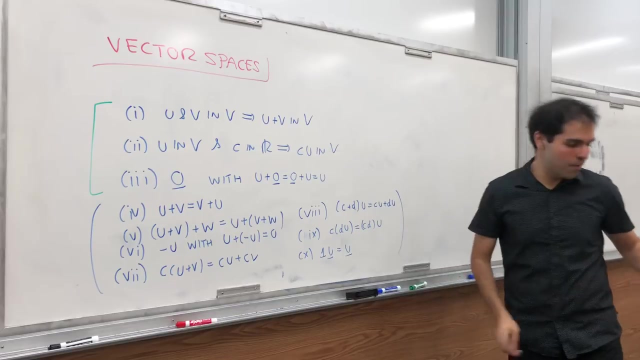 a vector u and you scale it by C, then the resulting vector should still be in your vector space. and lastly, there's also a zero vector that does nothing, namely if you add u to zero, you still get u. okay, but again, today is not much about the definition. it's really about examples. so let me start. let me give you. 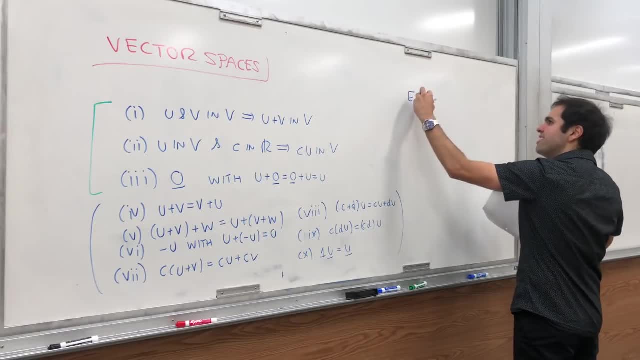 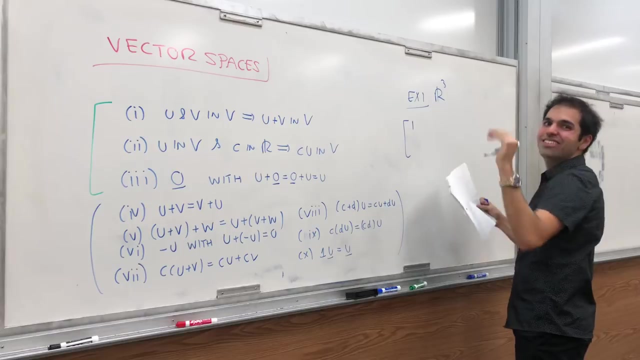 a bunch of examples. so first example: you've been dealing you for your life. probably it's Rn or for example, R3.. technically should be infinitely many examples, but yeah, but for now just maybe a basis of examples. think of it this way, and why is it a? 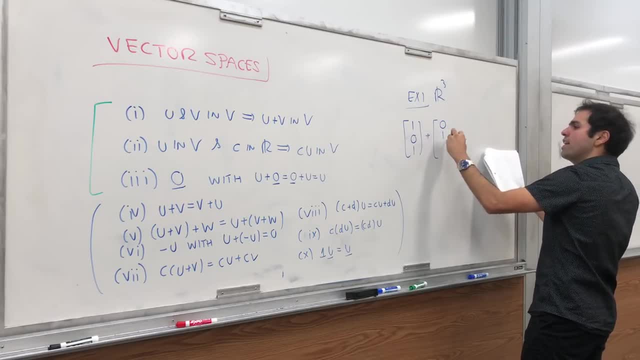 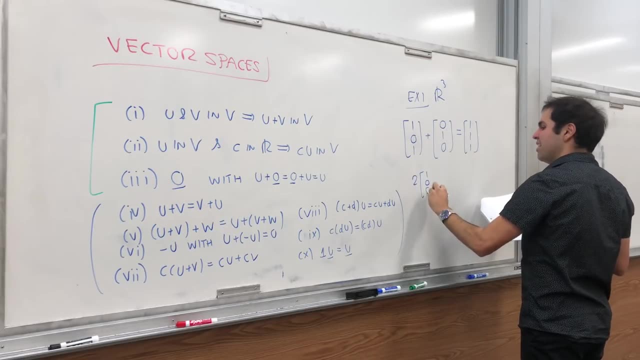 vector space. well, look, if you add two vectors in R3, you should get a vector in R3, and you know if you scalar multiply vector. then if you add two vectors with a vector like that, you get R3. so why does that matter? if you add two vectors in R3, you should get a vector in R3, and you know if you. 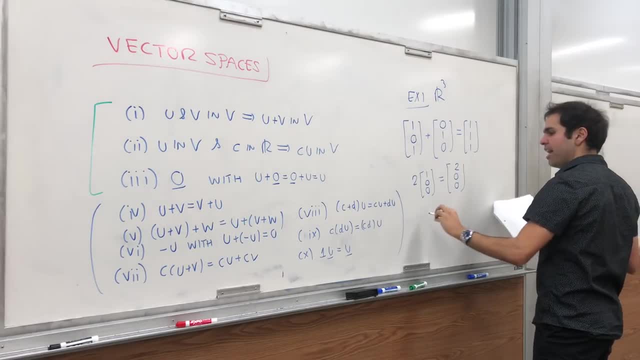 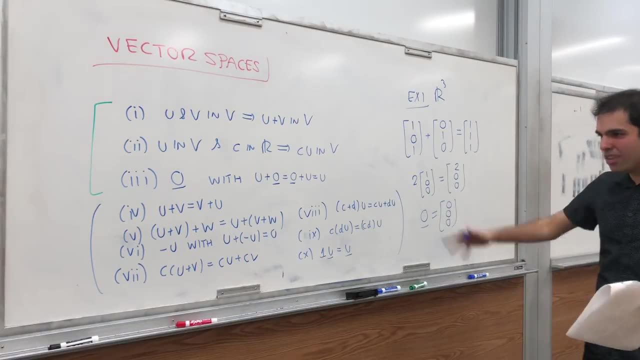 then you get two times that vector. And lastly, what is the zero vector? It's zero, zero, zero. So the first three properties hold and you can check that all the other properties hold as well, but this is left as an exercise to the reader. 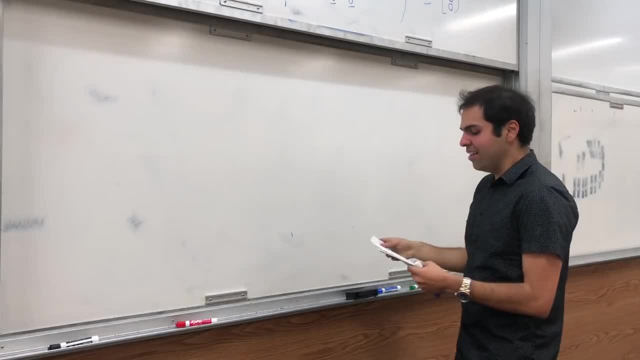 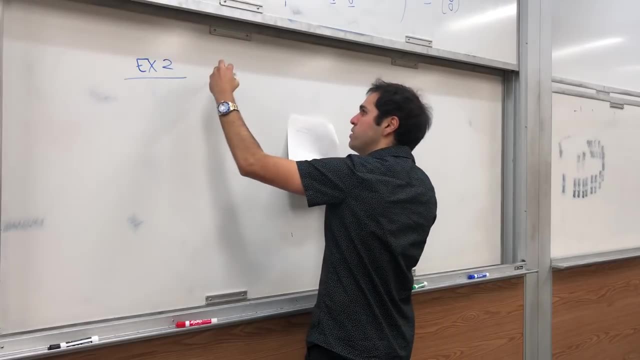 Okay, so that was example one, so 24 to go Well, and, as I said, more generally, Rn. but also another example you've been dealing with are matrices. so take M two by two, which is two by two matrices. 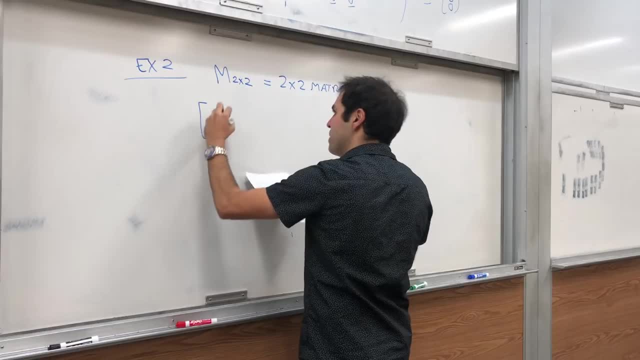 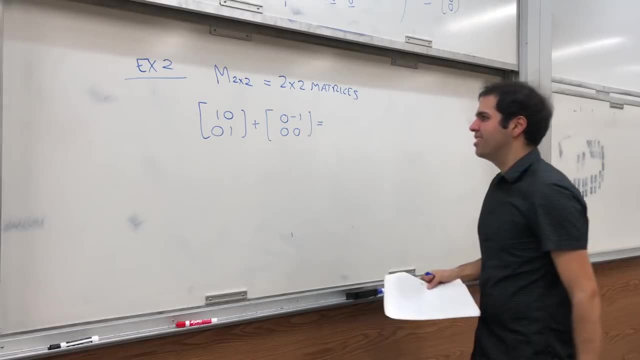 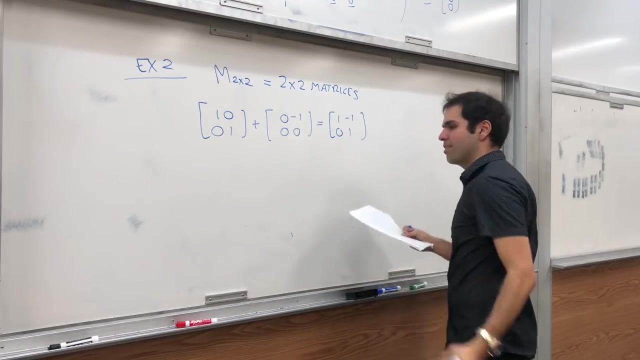 And indeed those are also another example of a vector space, because if you add two, two by two matrices, well, you don't get a monster, you get another two by two matrix, One minus one, zero one. And if you scale or multiply, 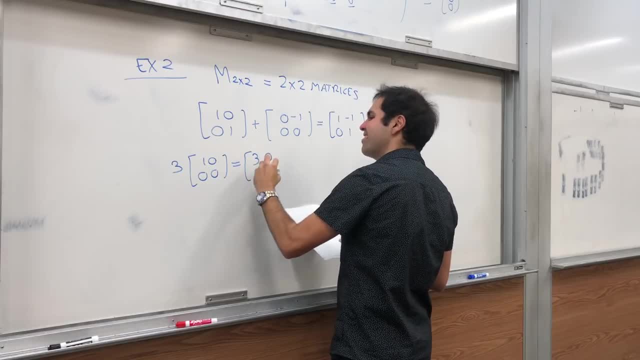 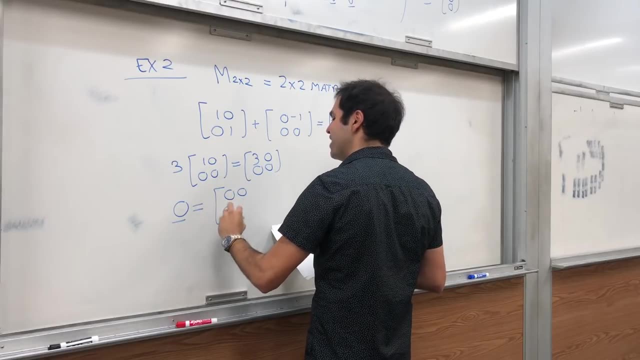 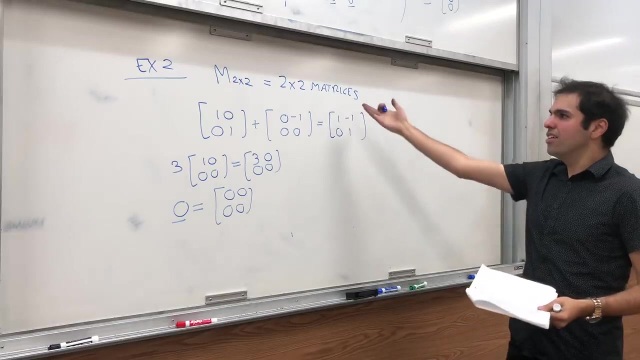 a two by two matrix. guess what? You get another two by two matrix. And what is the zero vector here? Interestingly, it's the zero matrix, because if you add any matrix to the zero vector, you still get that matrix. So two by two matrices are vector spaces. 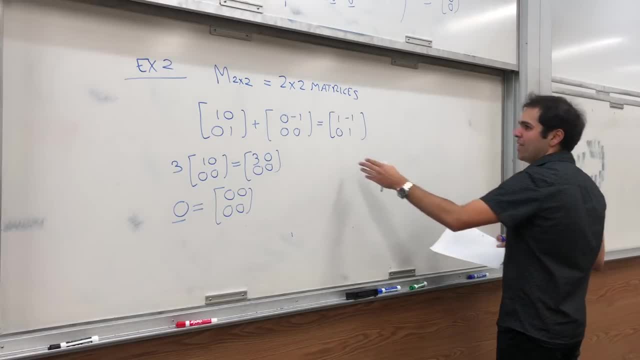 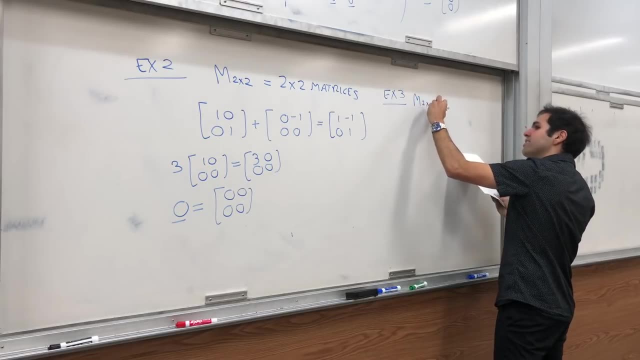 and in general M by M matrices, And it doesn't even have to be square, That's the nice thing. So third example: two by three you get three matrices. So for example: one, two, three, four, five, six. 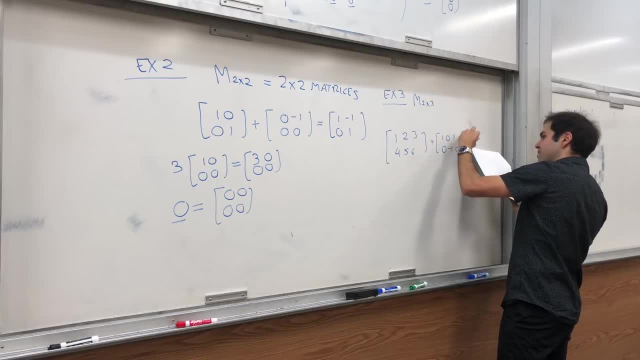 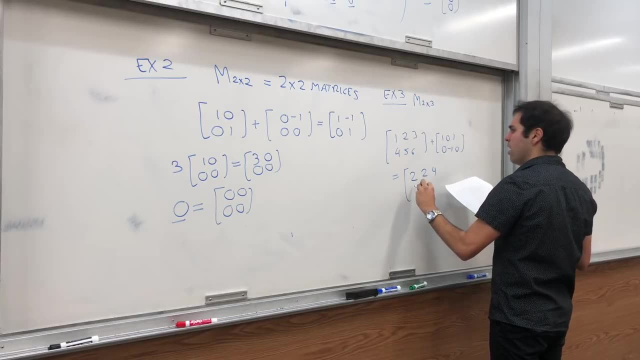 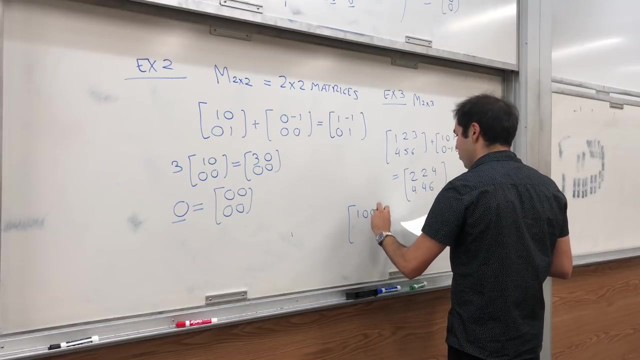 plus one zero, one zero minus one zero. You can add two matrices of the same size and you get two, two, four, four, four, six. And you can also scale or multiply a matrix: One zero, zero, zero, one zero. 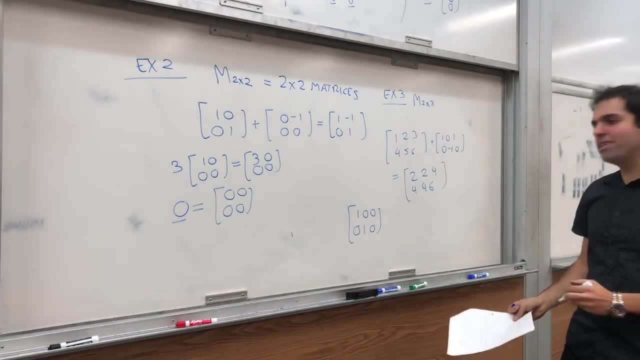 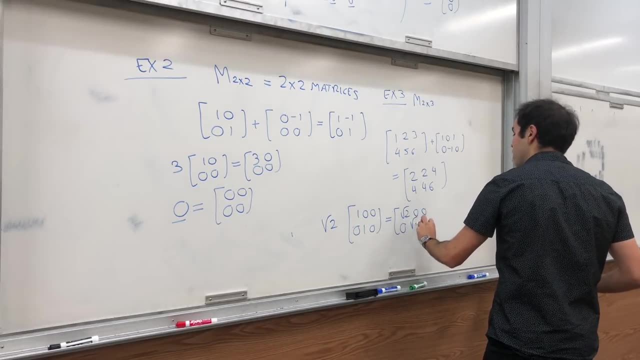 And I just wanna emphasize this number doesn't have to be, or doesn't have to be, an integer. You can scale or multiply by square root of two, And if you do that you still get a two by three matrix. So that's fine. 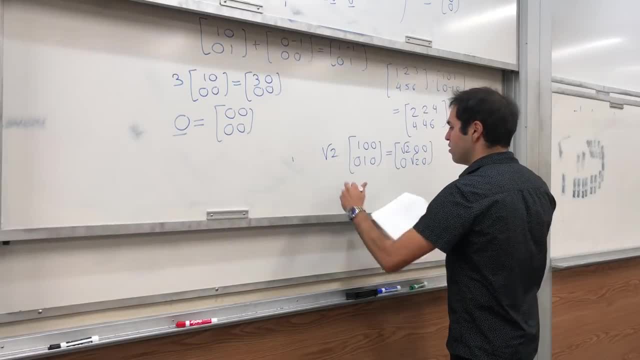 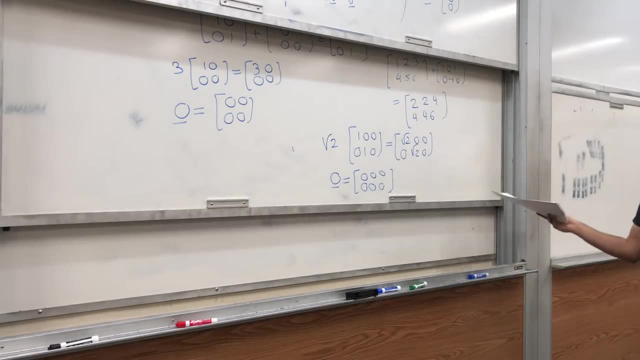 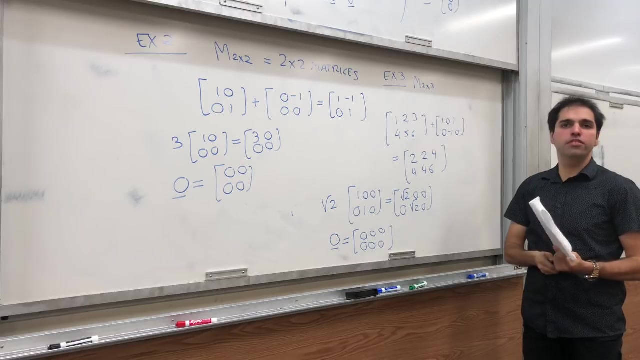 And you can check the other properties hold. And the zero vector, in this case also, is a zero matrix, a matrix that does nothing, And so also more generally you can get M, M by N, So the space of matrices of size M by N. 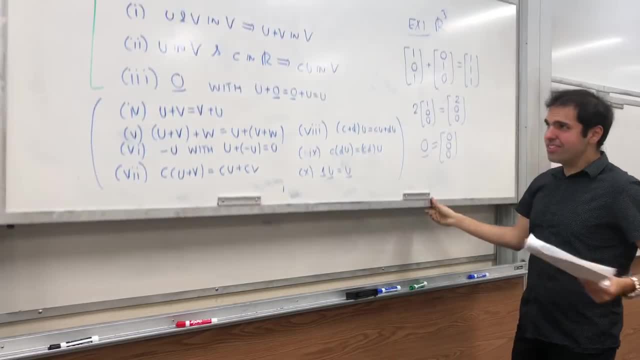 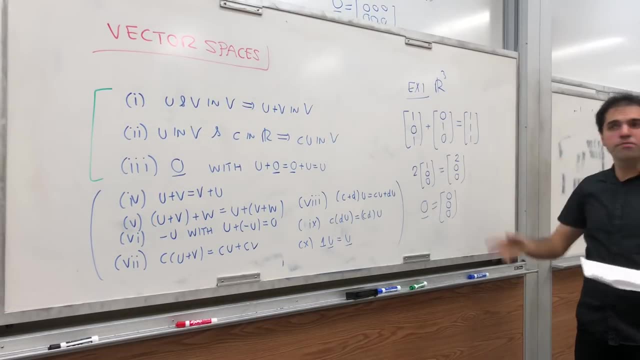 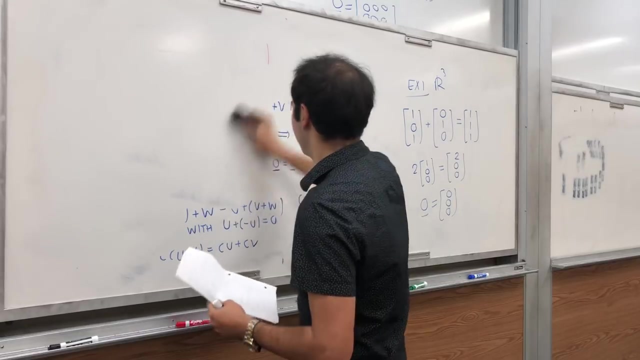 Okay, good, And so it's interesting. here you will think of vectors. They can be actual vectors in RN, but also matrices could be vectors And, even weirder, you could have polynomials being vectors. So the next phase is just the set of polynomials of. 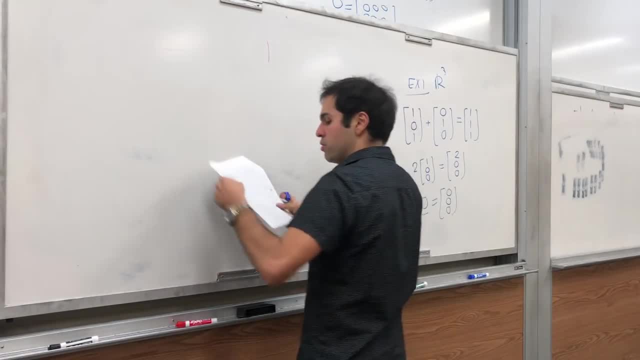 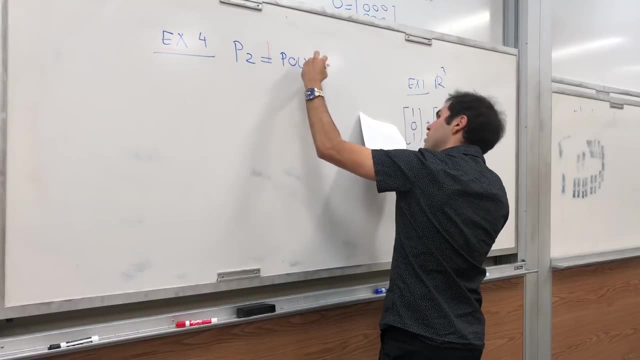 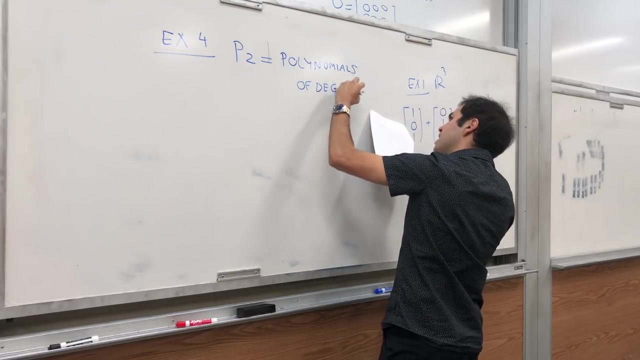 let's say of of degree less than or equal to something. So example four: let's call it P2.. And it's a polynomial of degree, of degree less than or equal to two. So polynomials with real coefficients of degree less than or equal to two. 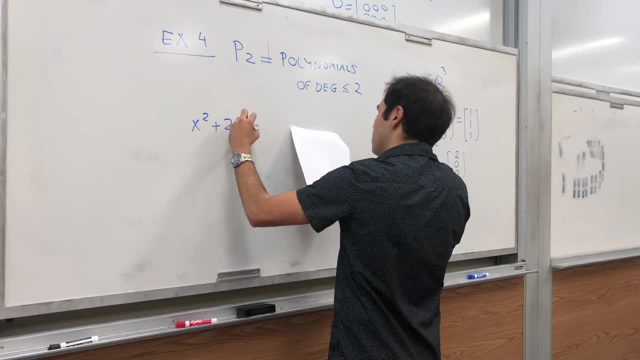 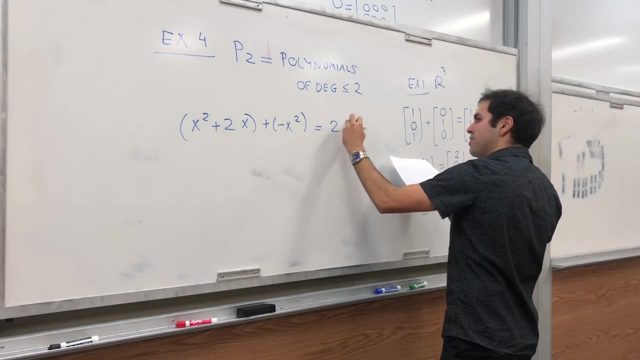 And indeed you can add those right. If you take X squared plus two X and you add I don't know, minus X squared, then you get two X. And this is very interesting because you might be tempted to say: 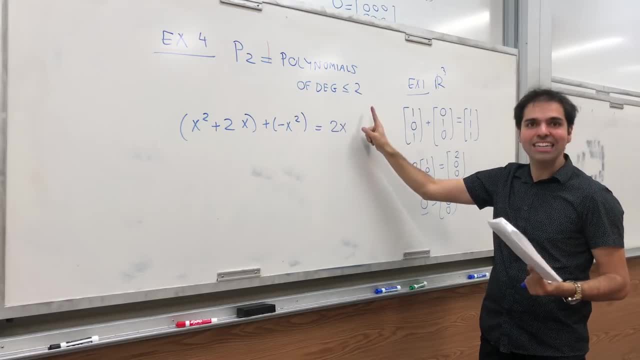 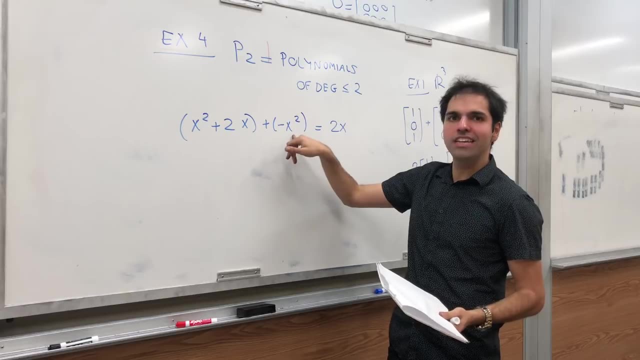 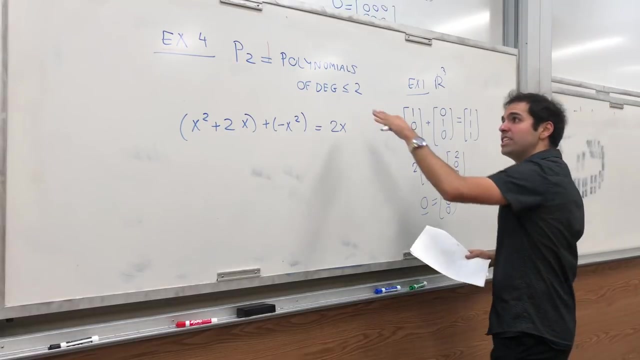 what about the set of polynomials of degree exactly two? Well, technically that's not a vector space, because if you add those polynomials of degree exactly two, you don't get a polynomial of degree exactly two. Here the degree is one. 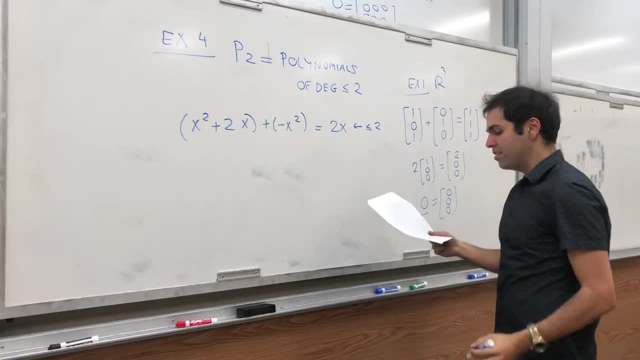 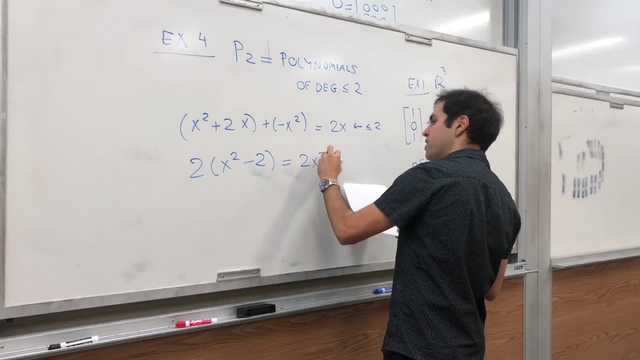 which is okay because it's less than or equal to two. So that's fine. And also you know you can scale or multiply such a polynomial and get two X squared minus four. So basically all the operations you've done before. 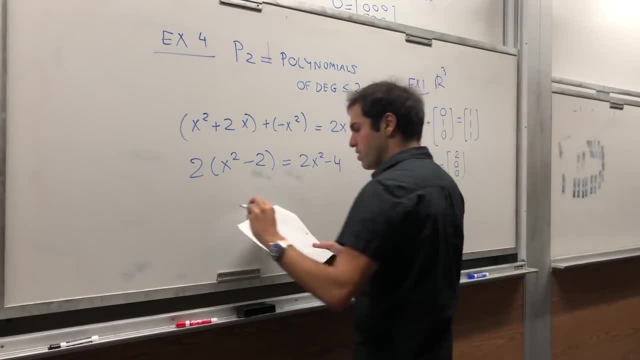 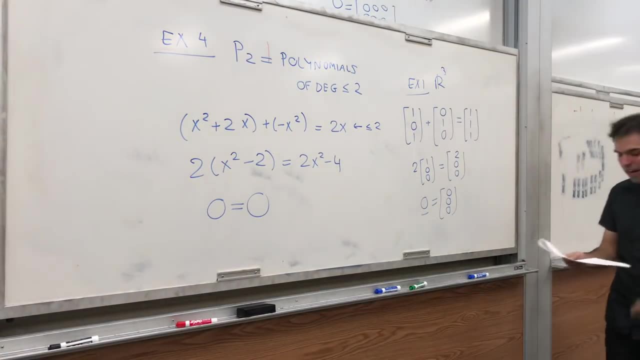 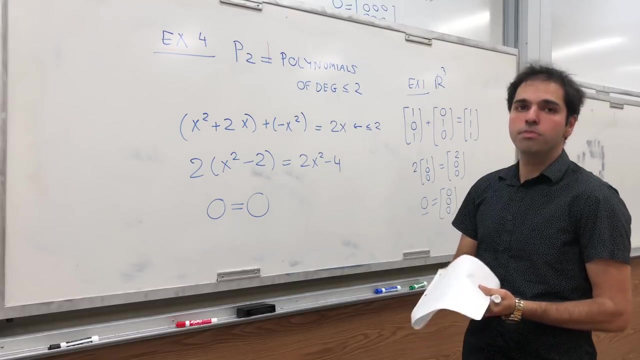 but put in a more general context. And what is the zero polynomial? We're literally the zero function, the polynomial that's zero everywhere. And of course we have P2, there's nothing special about two. You could have Pn, You could have the space of polynomials of degree. 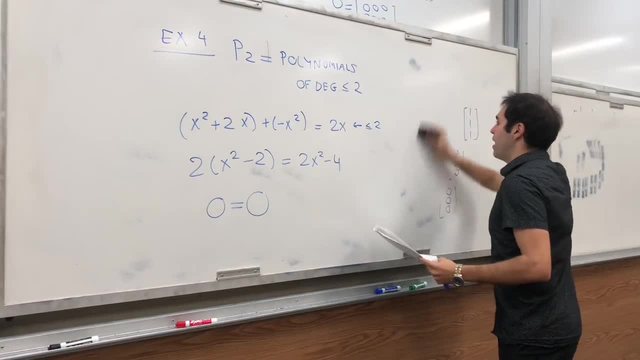 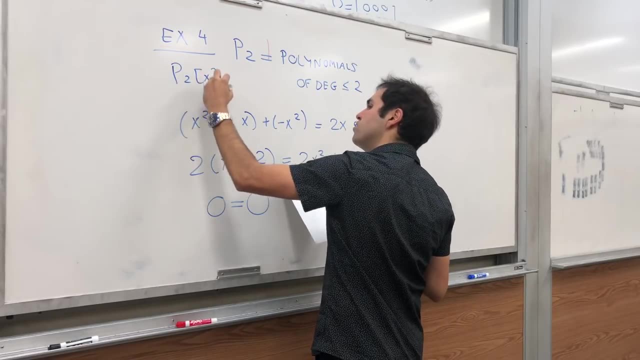 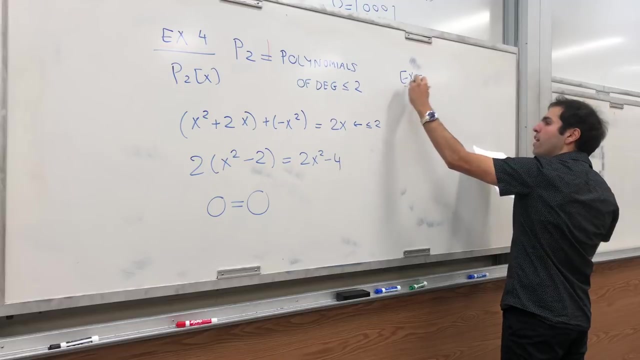 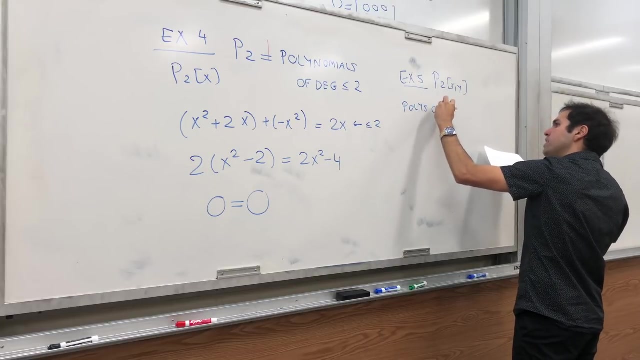 less than or equal to n And, by the way, so sometimes this is called P2X because it's a polynomials with variables X. You could have it with any number of variables. So take example five P2XY, which is polynomials of degree less than or equal to two. 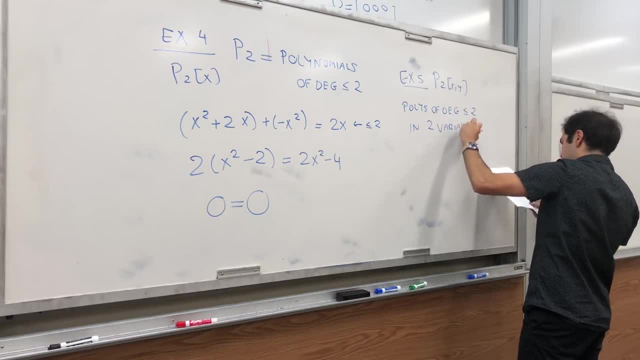 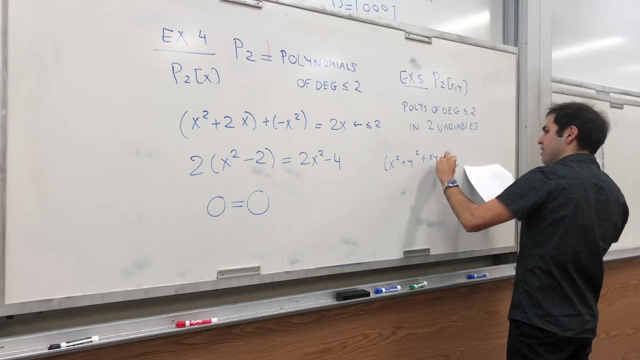 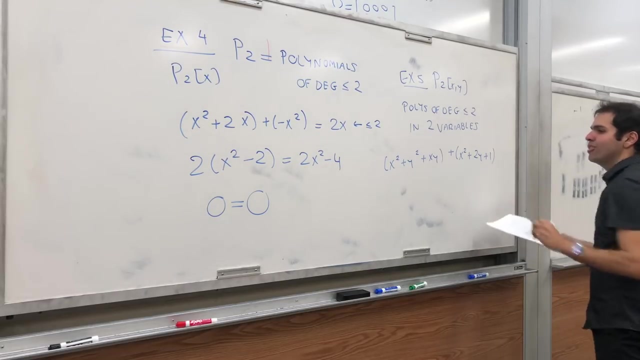 In two variables, Because in D, if you, for example, add X squared plus XY plus X squared plus Y squared plus XY, and you add it to X squared plus two, Y plus one, So it's a polynomial of degree less than or equal to two. 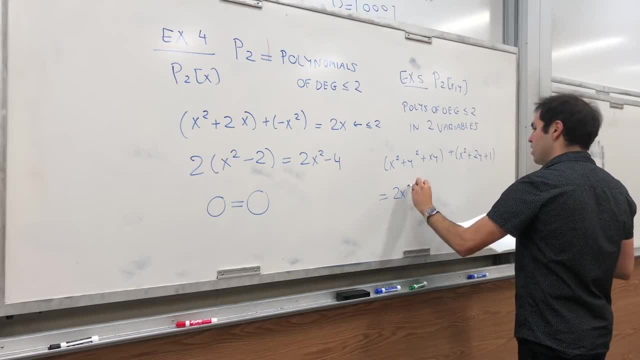 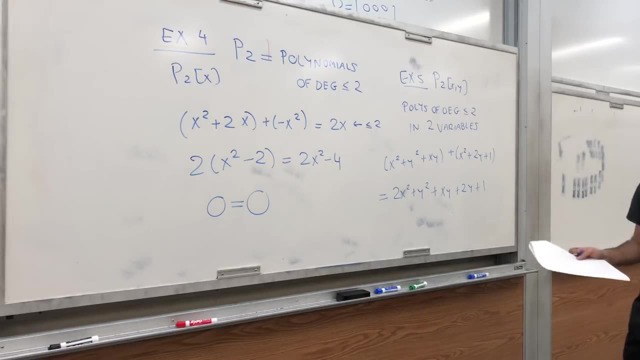 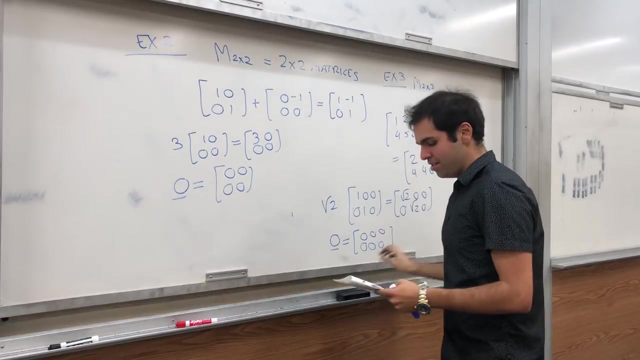 in two variables, You still get a polynomial of degree less than or equal to two in two variables: XY plus two, Y plus one plus one. all right, and you may guess. well, we did it with polynomials, which are functions. well, indeed, you could also have functions from R to R again, just to. 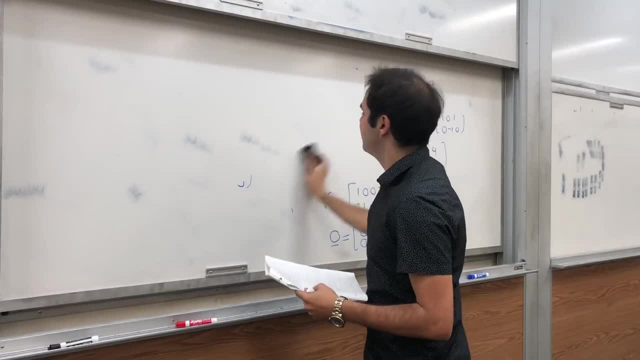 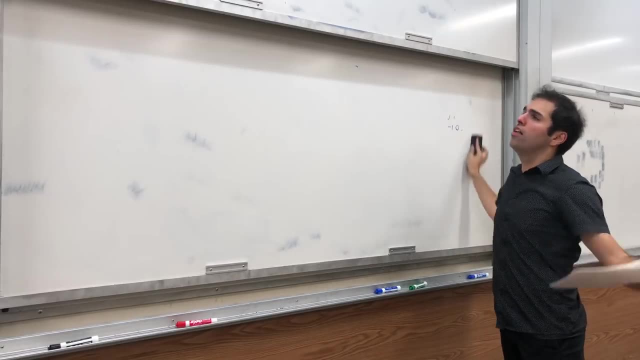 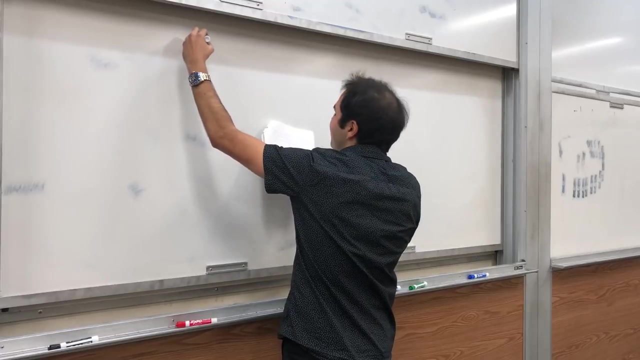 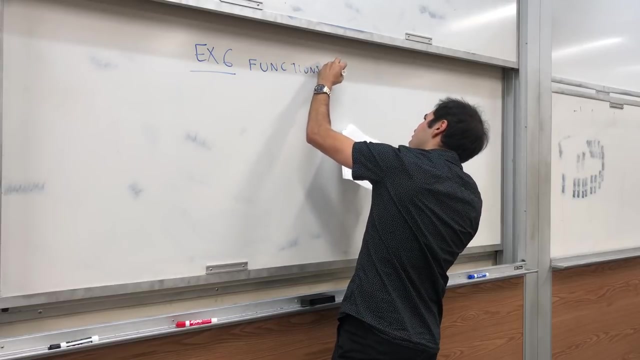 show you while you do. linear algebra deals with vector spaces. it's such a rich theory because all the stuff we say in this course applies to all those spaces all together. how amazing is that? so you're like killing 25 flies with one stone here in this case. so example: six functions from R to R. for example, take f. 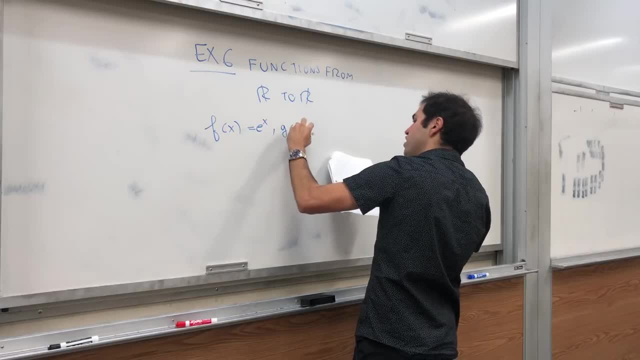 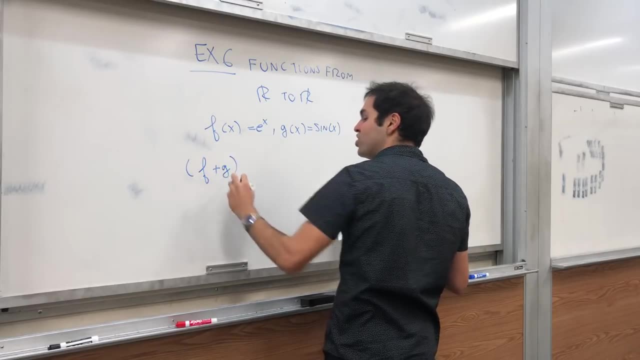 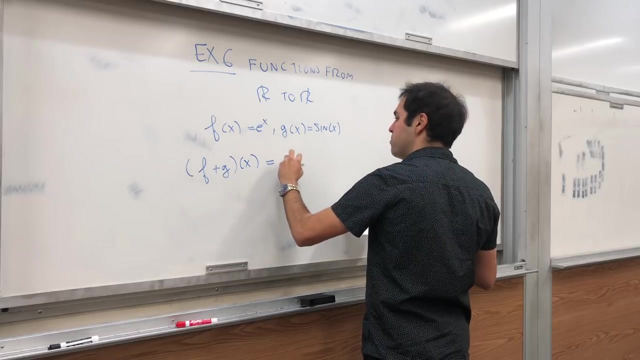 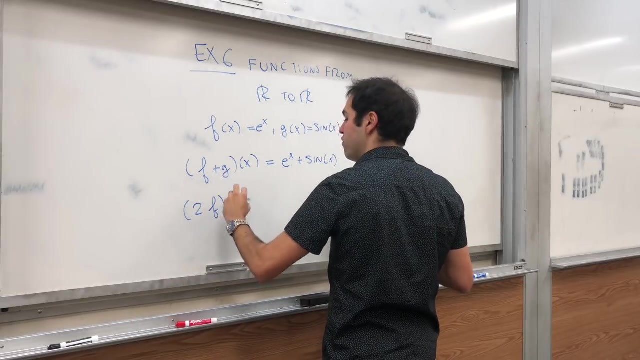 of X is e to the X and G of X is sine of X. well, you can add two functions: what is F plus R plus G? it's the function whose input is X and whose output is the sum. so e to the X plus sine of X. or you also have, you know, two times F of X, which is just in. 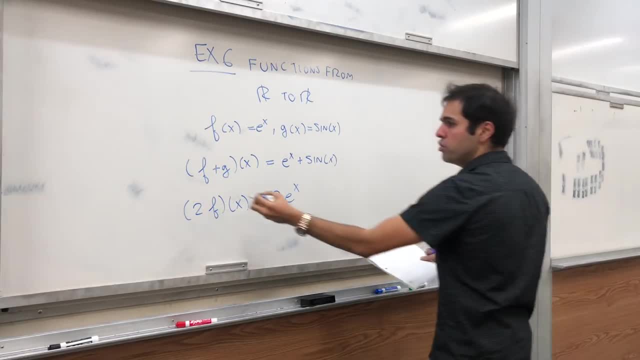 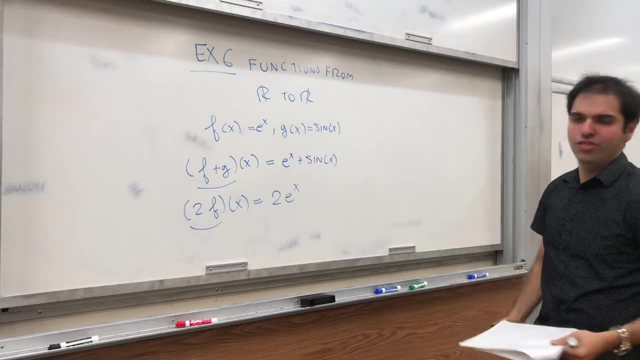 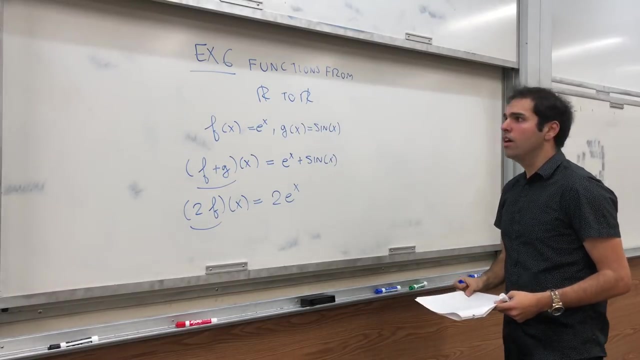 this case 2 e to the X. so the point is you can define F plus G, you can define a constant times F and the zero function is the zero function and the. there's nothing special from R to R. you can replace it with any variable, I mean. 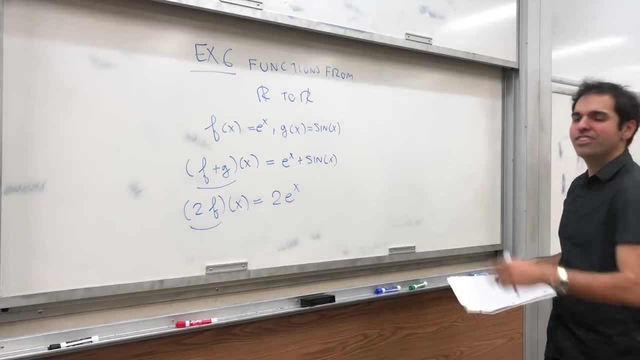 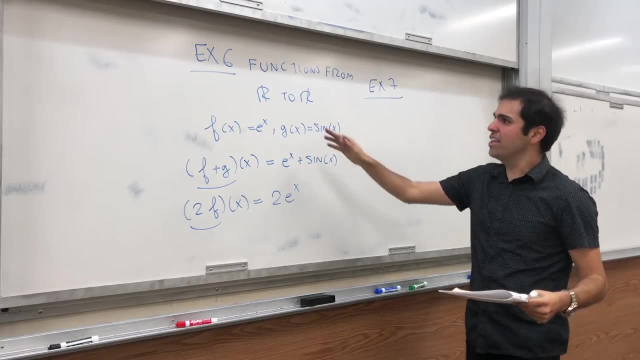 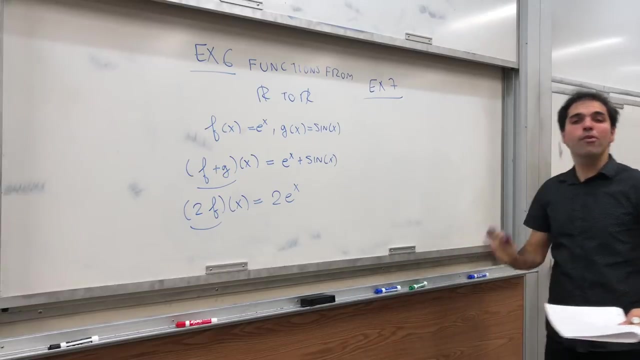 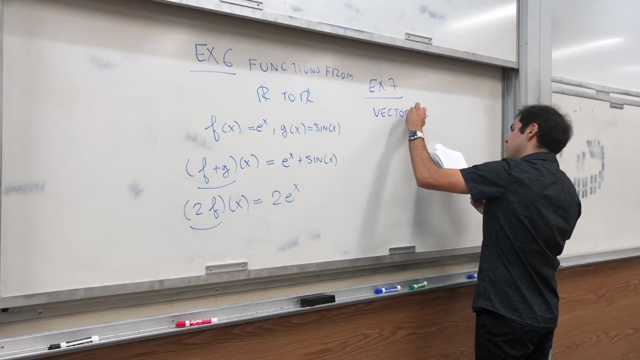 any interval. you can have continuous functions, differentiable functions, whatever, and in fact not only can you have functions from R to R, you can have functions from Rm to Rn, for example. one thing you dealt with: multivariable calculus. you can have vector fields in R3, for example the vector field F of XYZ, maybe e to the z, e to the X minus. 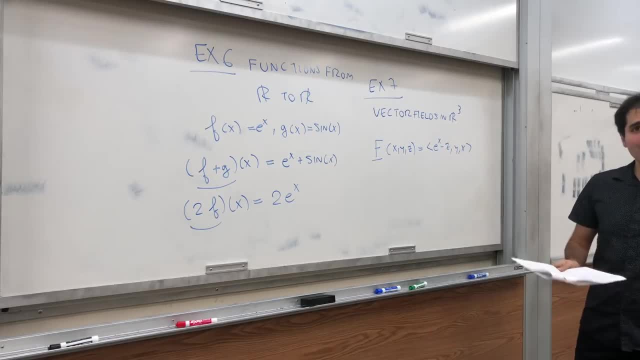 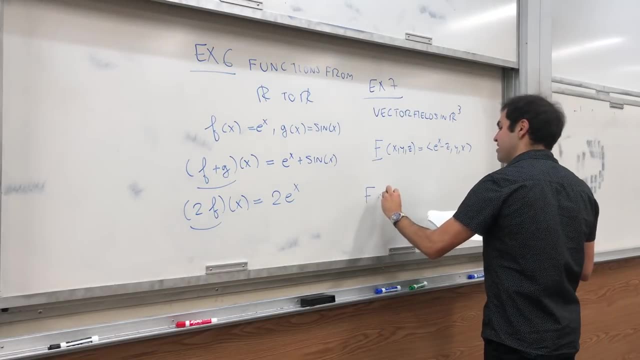 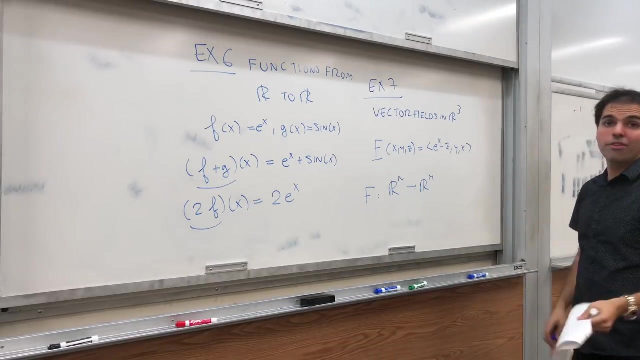 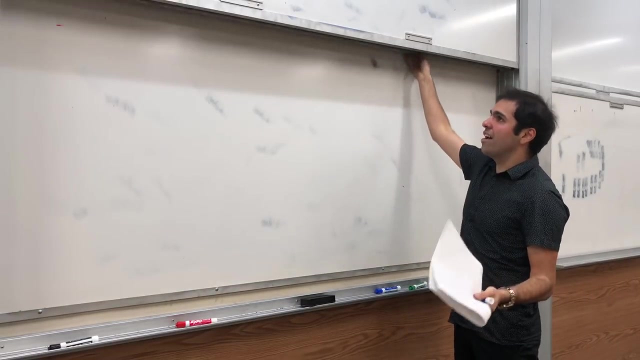 Z, y, X. so everything you've done in multivariable calculus you can define with linear algebra and more generally, as I said, functions from Rn to Rm, so maybe 2 inputs and 3 outputs. that's what's here also works, as I said, really, really rich. and going back to calculus, we could also: 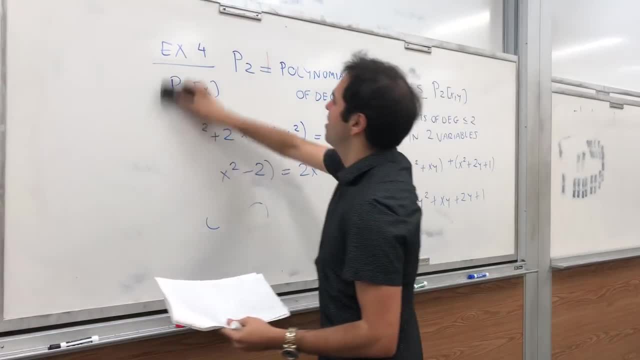 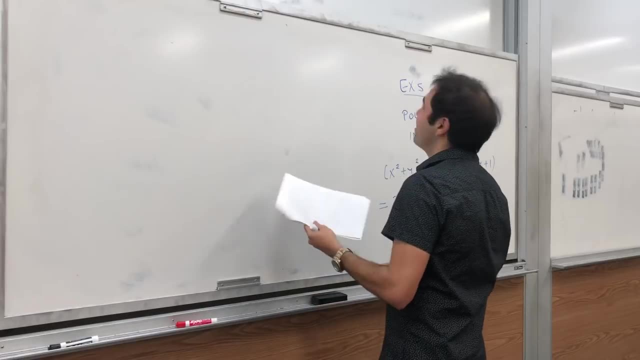 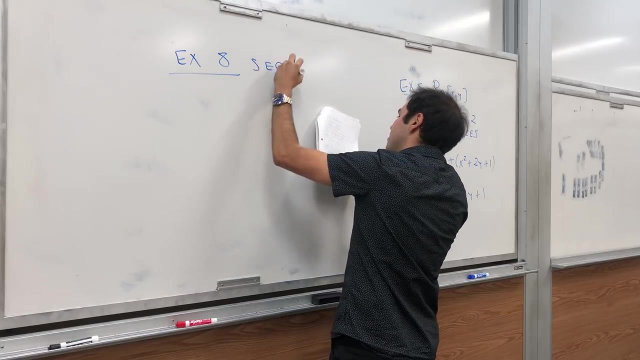 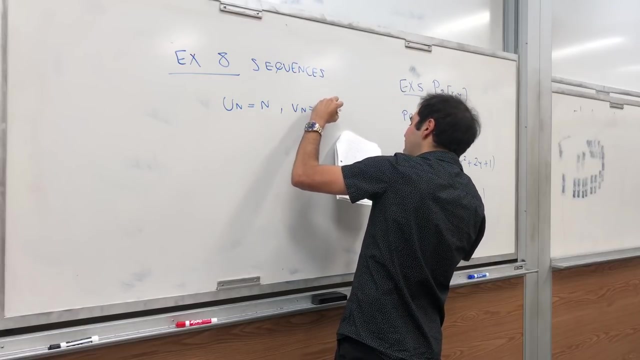 have discrete functions which are sequences. basically, all of calculus is included in the study of linear algebra, which, okay, I'm simplifying a little bit because not everything is linear, but anyway. so we can have sequences. for example, if un is the sequence n and vn is the sequence minus 1 to the n, then 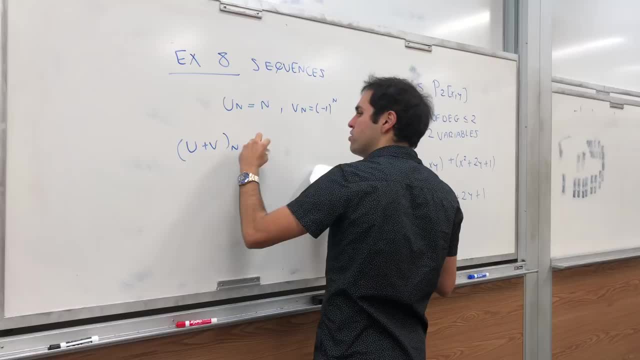 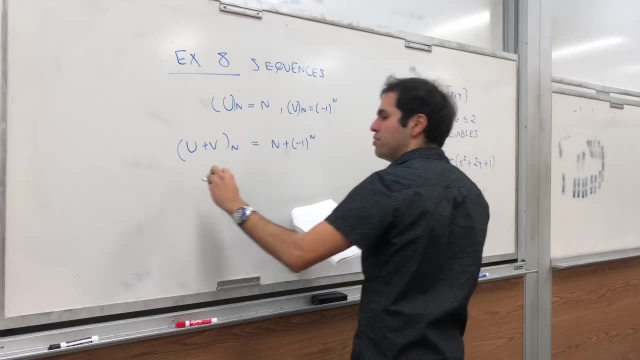 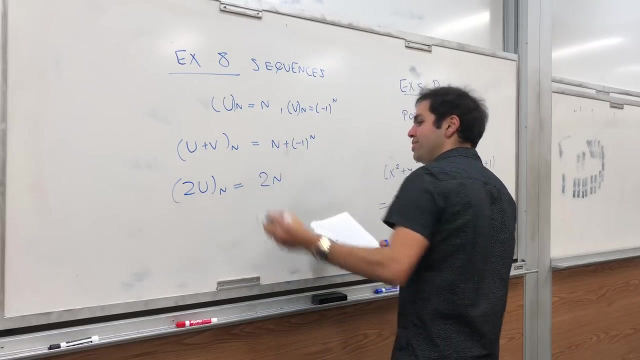 what is u plus v? the sequence is just u plus vn, it's just n plus minus 1 to the n. let me write it this way, and then also two times the sequence u: n is just 2n, just the sequence 2n. so sequences, you can also write them, you know, as vectors. 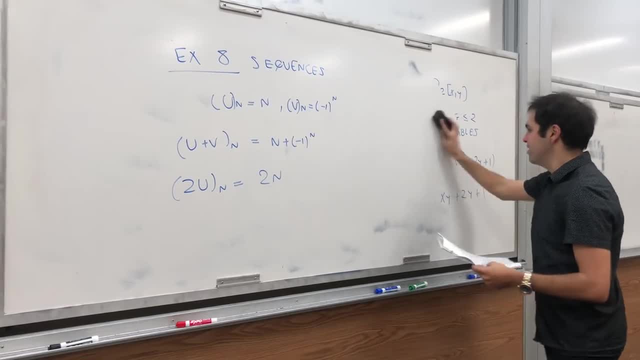 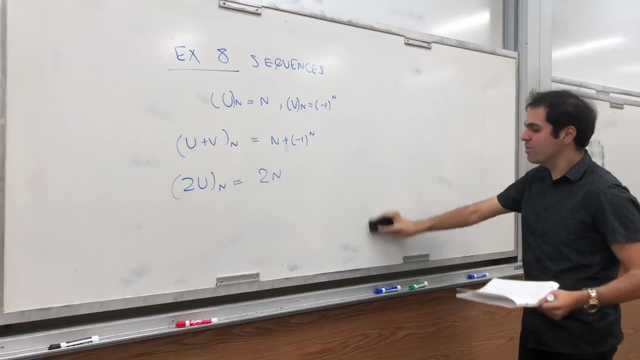 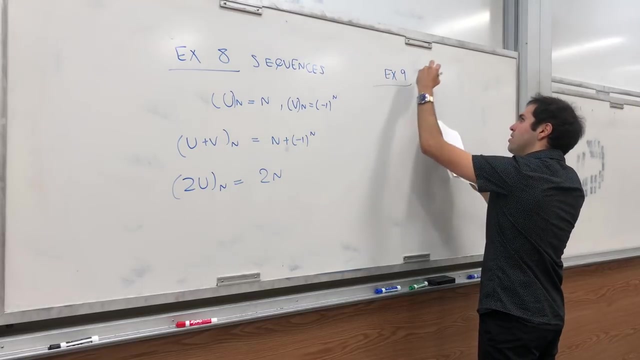 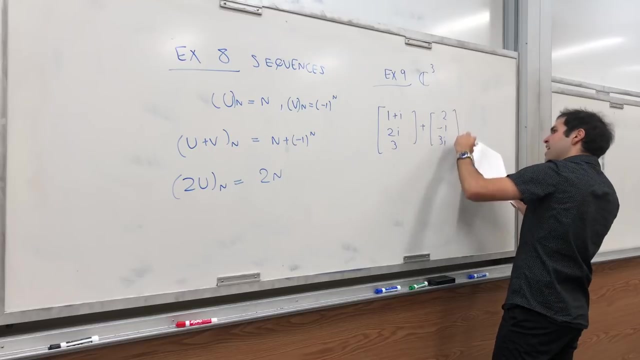 spaces and the zero vector is the zero sequence and moving on. so you could have all vector spaces, not only over the real numbers. you can have vector spaces over the complex numbers. so you can take the complex space, so CN, for example, or c3. in this case you can have the vector 1 plus I, 2, I, 3, you can add it to 2 minus 1, 3, I. 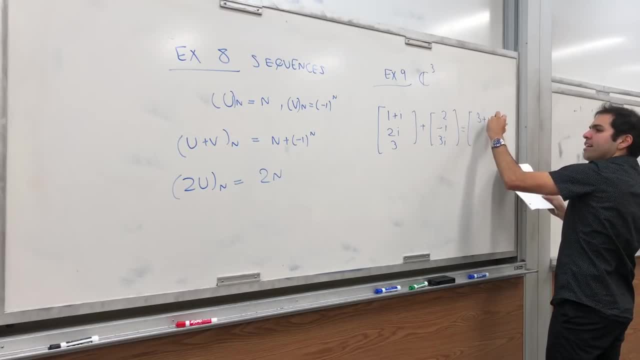 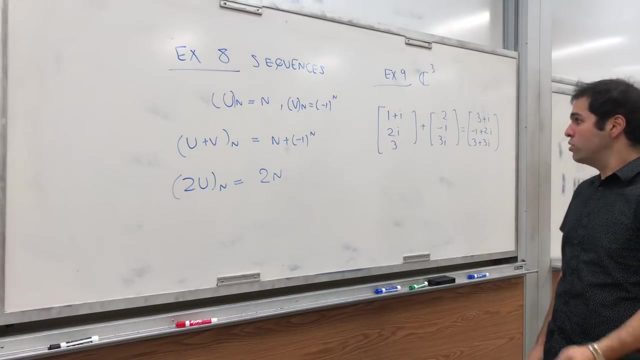 when you get, you know, 3 plus I and then minus 1 plus 2 I and 3 plus 3 I. the interesting thing is well the constants you can, depends what you're fixing first. you could have your constants just be a real numbers. you could have your constants just be a real numbers. 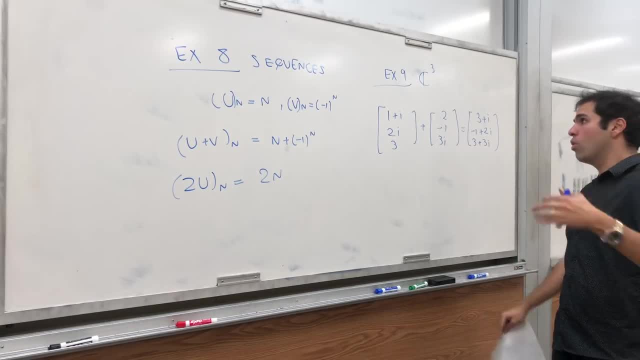 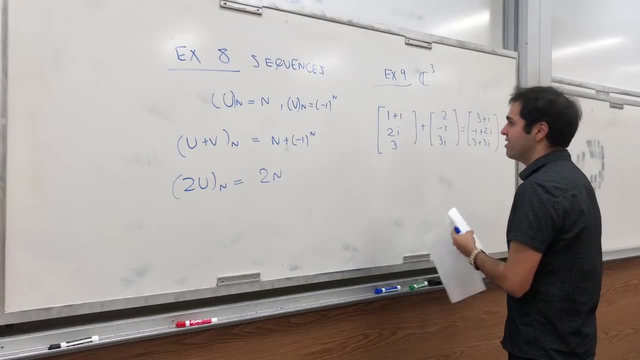 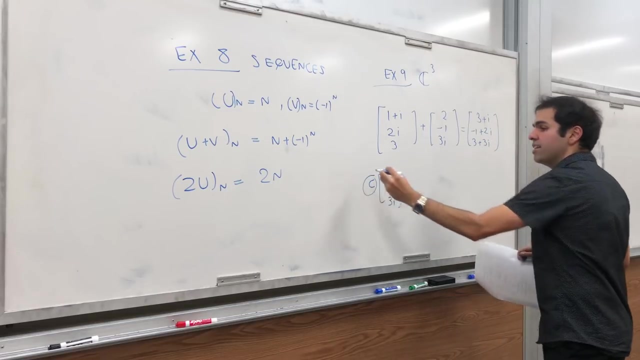 and it becomes a vector space over the real numbers. or you could have vector space over the complex numbers, in which case your constants see as in C times this: C times I, 2, 3, I, this C if your vector space is over the real numbers, C. 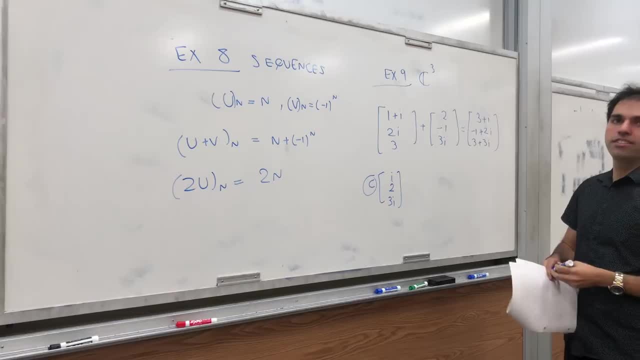 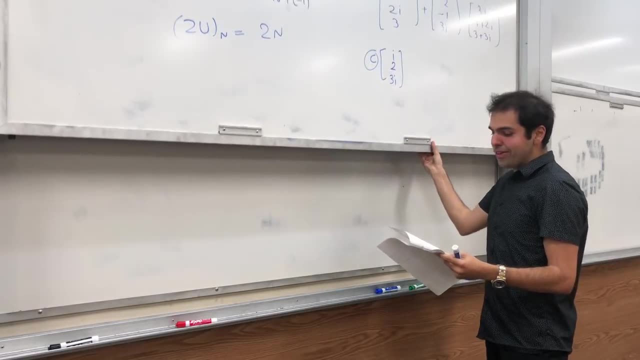 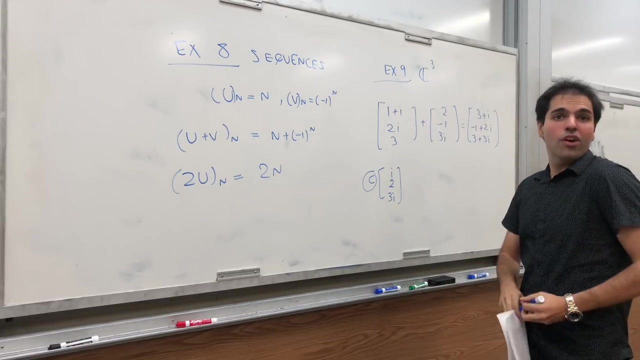 is real if your vector space is over the complex numbers. and C is complex, but in both cases it becomes a vector space. that's a cool thing, and also so dealing with calculus again. so we did sequences, we did polynomials. well, we could also have Taylor series right. so power series, which are just 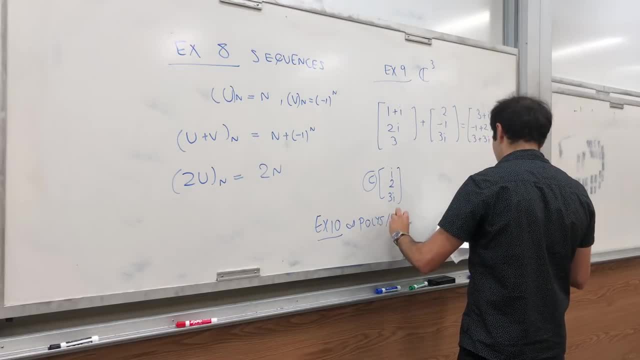 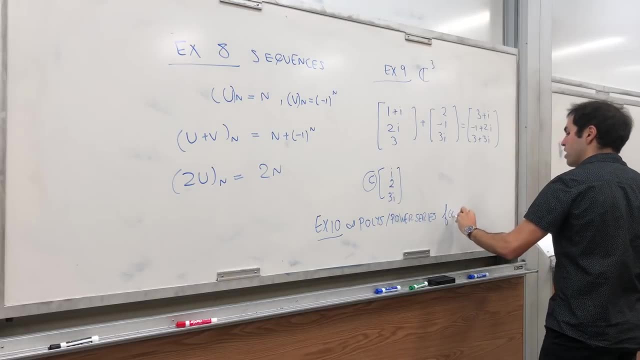 infinite polynomials or formally you can add them up and you get a vector space. so 1 plus X plus 2x squared plus 3x squared times the vector space. so this is it: X, Q plus dot, dot, dot dot. This is a vector in this vector space of power series. 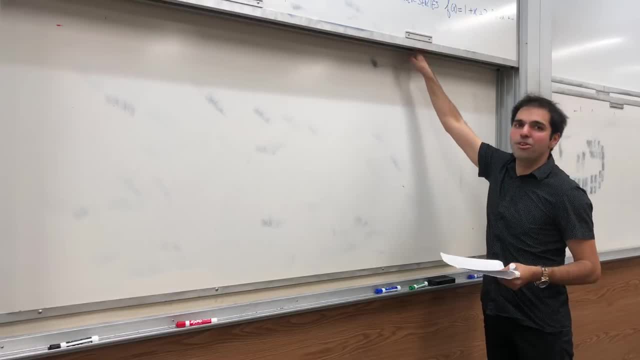 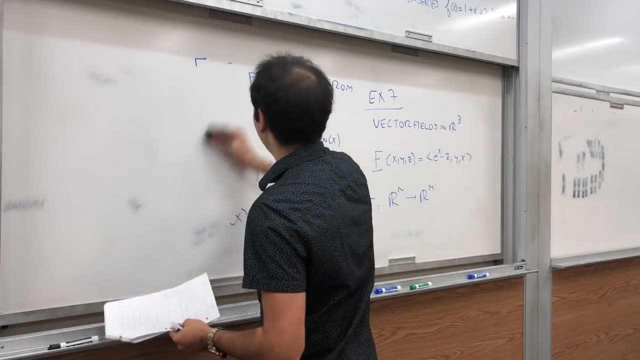 And we're not dealing with convergence issues. So we're not talking about convergent power series, but then it might also be a vector space, the convergent ones, Because if you add two convergent power series, you get another convergent power series. 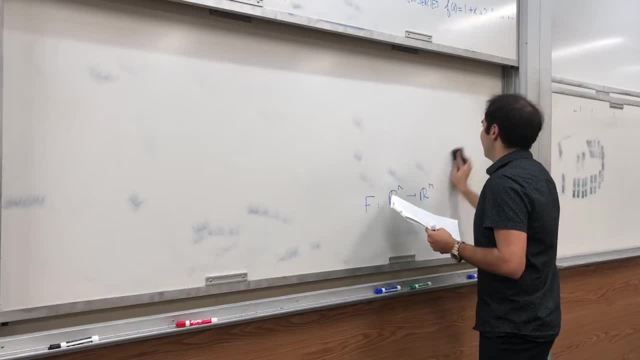 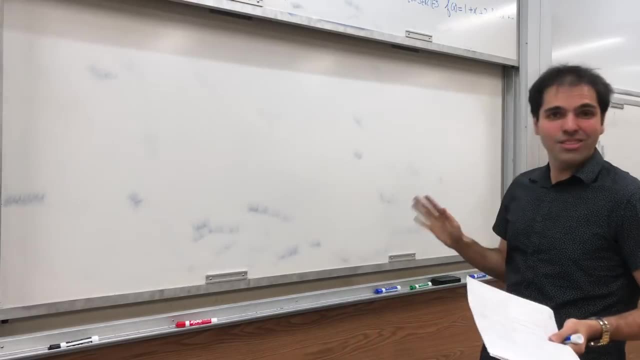 Same with scalar multiplication, At least if it converges on the same interval and stuff, then it's okay, Okay. and then there's some fancier examples and don't laugh at that. So, and I'm sure some people are like 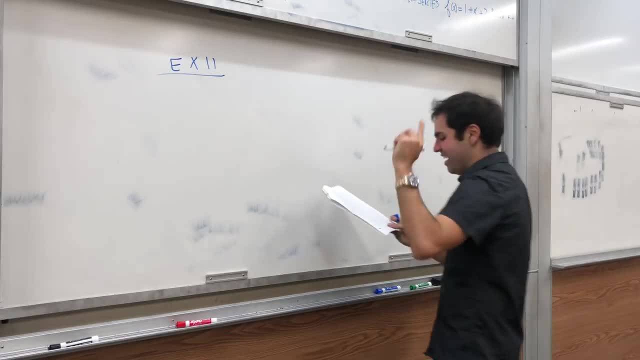 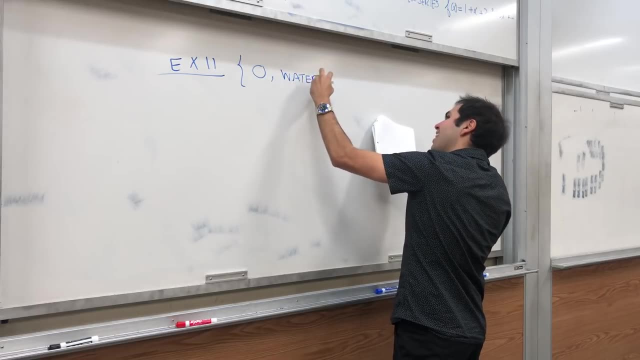 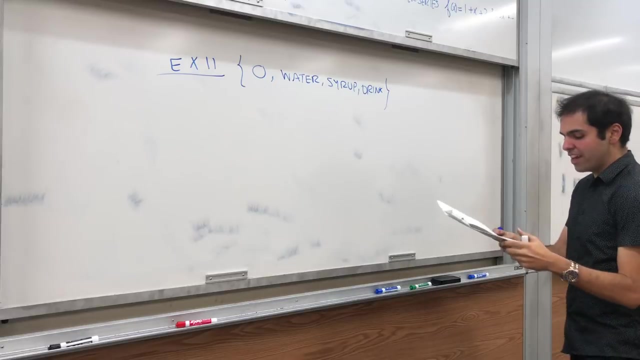 this is not a vector space, But in my case it is okay. So take the zero vector, so nothing water and then syrup and drink. Just want to show you. it can be very abstract, but it could be a vector space. 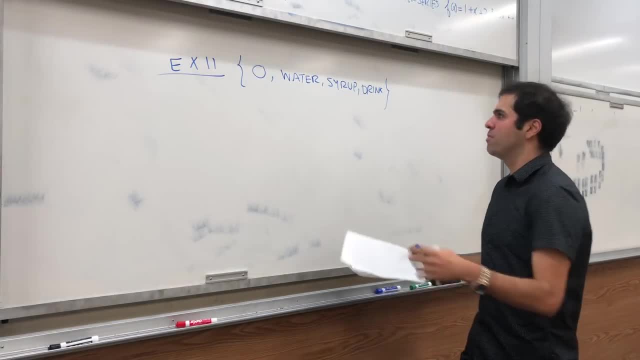 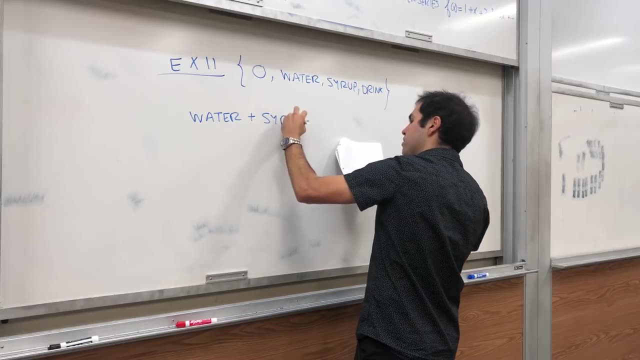 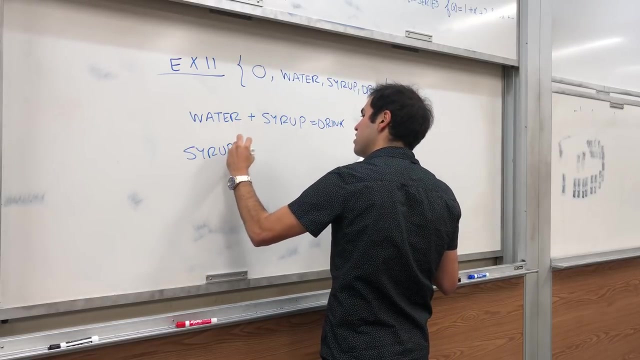 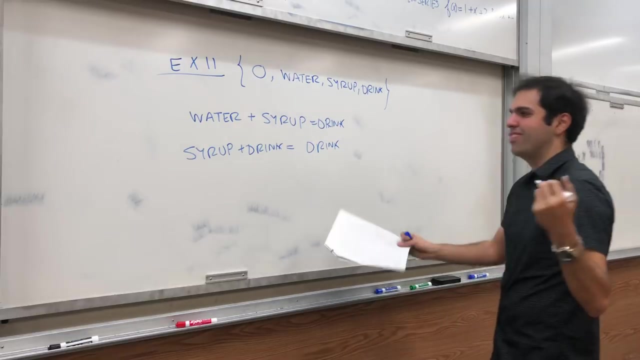 And, in particular, how do you define your addition and your scalar multiplication? Well, water plus syrup: If you add water and syrup, you get drink. Or if you add syrup and drink, you get a very sweet drink. So yes, in fact, syrup is the zero vector. 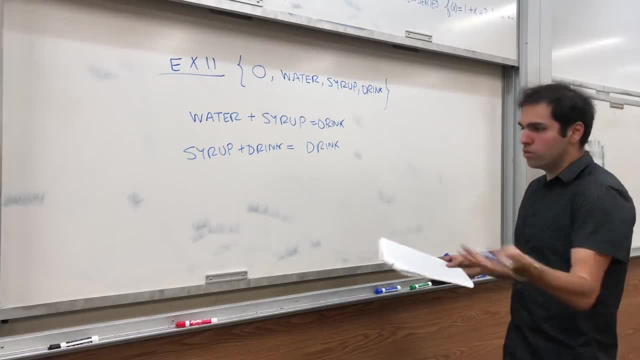 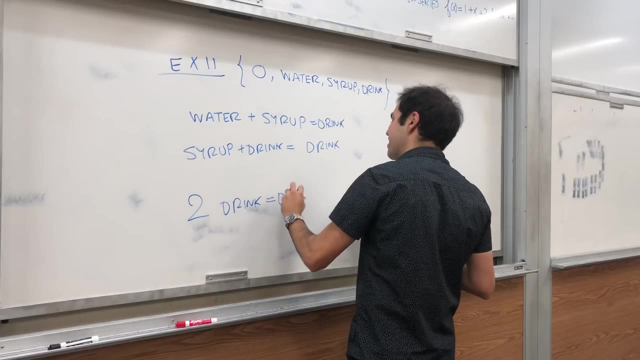 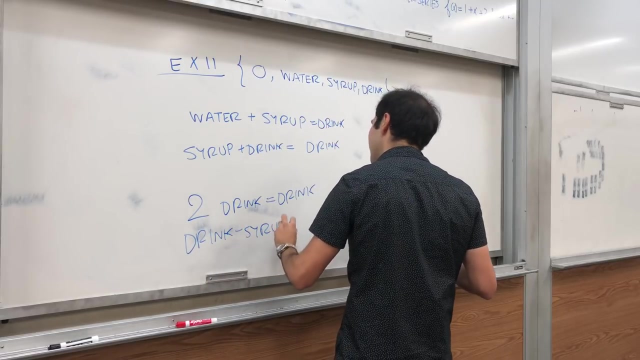 so this might be a very trivial vector space. But you could also, you know, scalar multiply. So two times drink- well, it's still a drink. Or drink minus syrup- well, it's just water. So it's a very silly vector space. 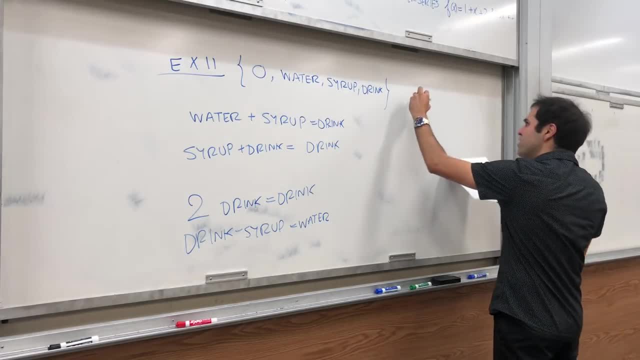 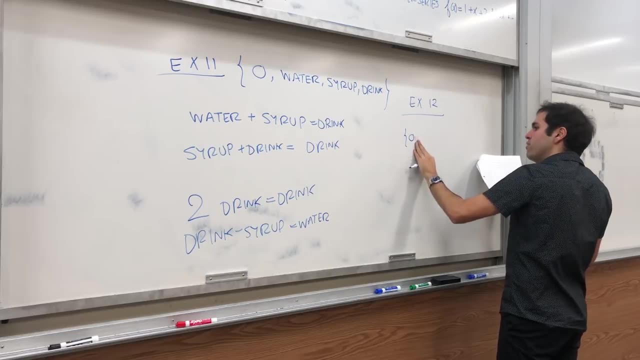 but I just want to show you abstractly. you can have that, But here's a more interesting one, Example 12, namely: just take the vector space zero one times 0, one, So you've 1 and 0 one squared. 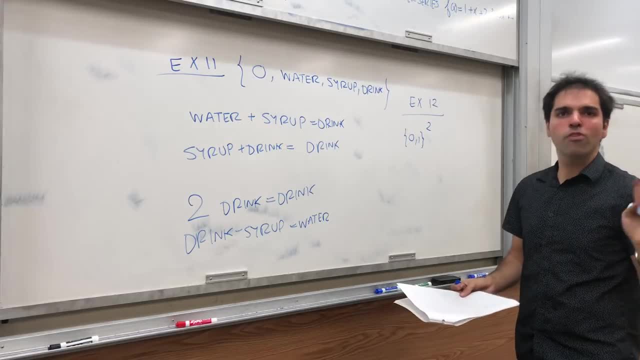 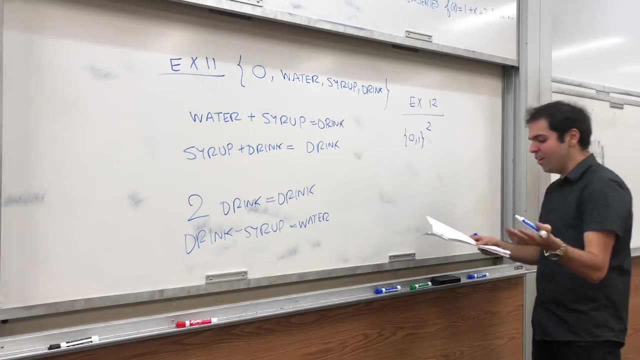 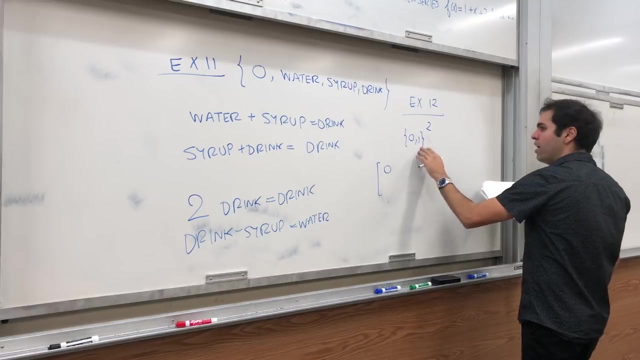 Careful this wouldn't be a vector space over the real numbers. It would be a vector space over some weird field which is just the field 0 one. And let me tell you how to add and scalar multiply vectors. Namely, it's 0 one with the convention. 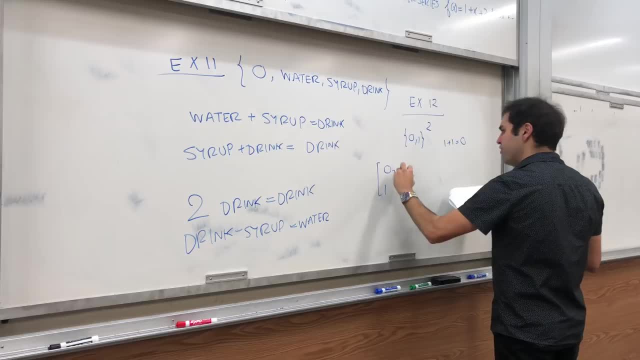 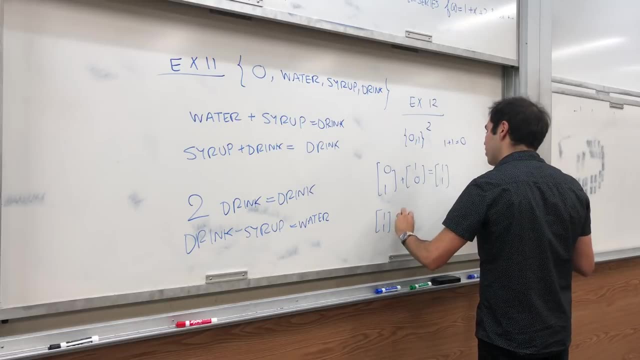 that one plus one is zero. So then if you add the vector and 1, 0, you get 1, 1.. But if you add 1, 1 and 1, 1, you would actually get the 0 vector. 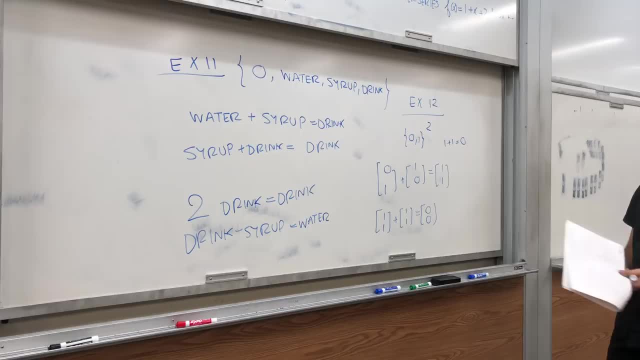 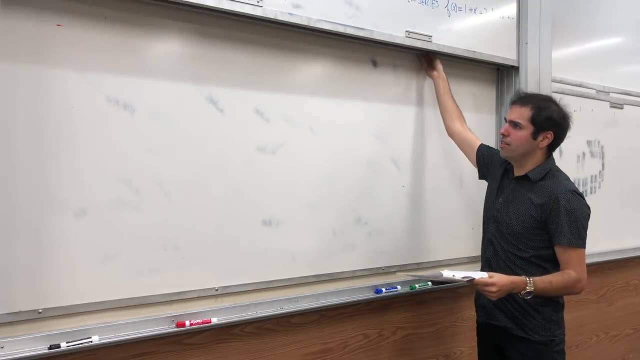 So in fact minus 1, 1 is just 1, 1, just by definition. So you could have those fancier vector fields and I think vector fields over, I think fp or something, And there are some really cool ones. 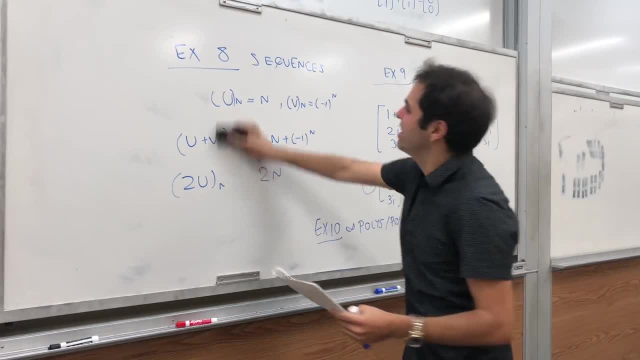 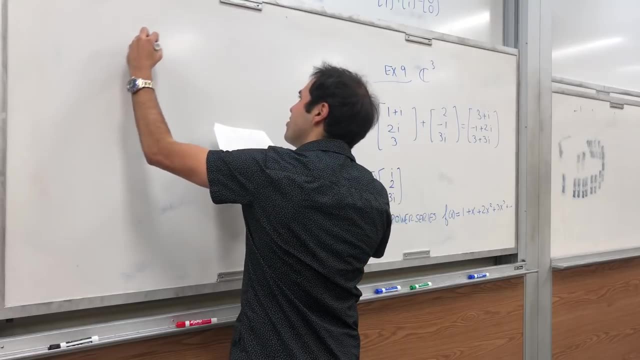 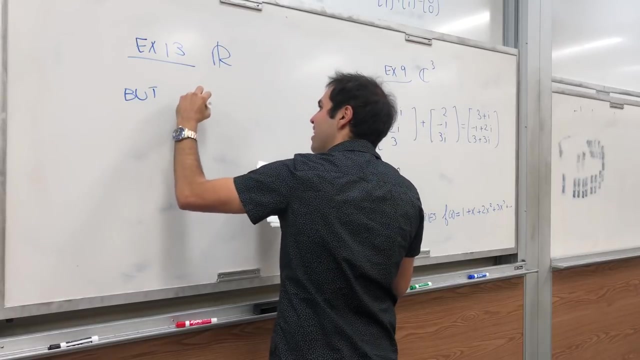 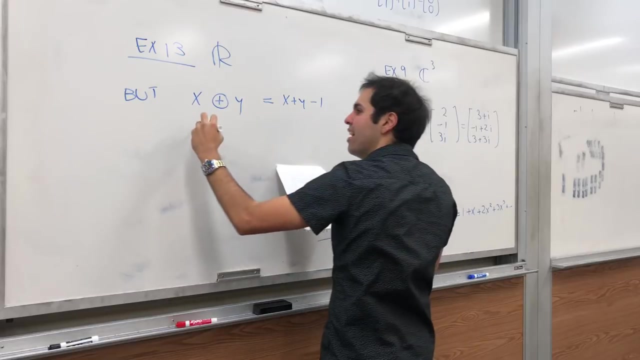 because sometimes addition and scalar multiplication isn't what you think it is. So let's do example 13.. So, halfway done, Let's take the real numbers. but you define addition as follows: x plus y is x plus y minus 1.. 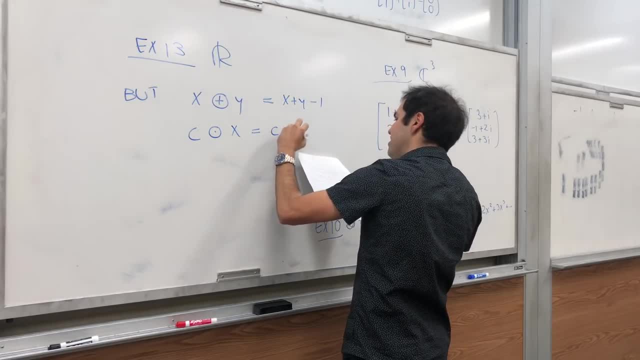 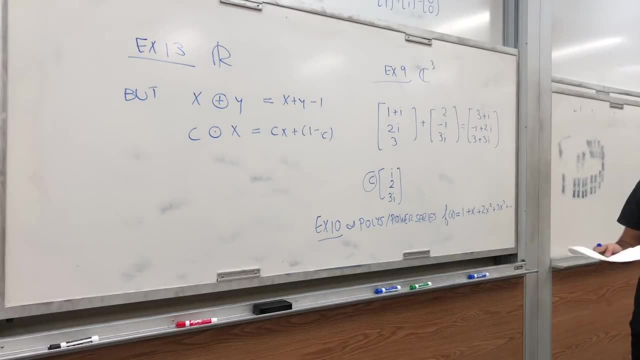 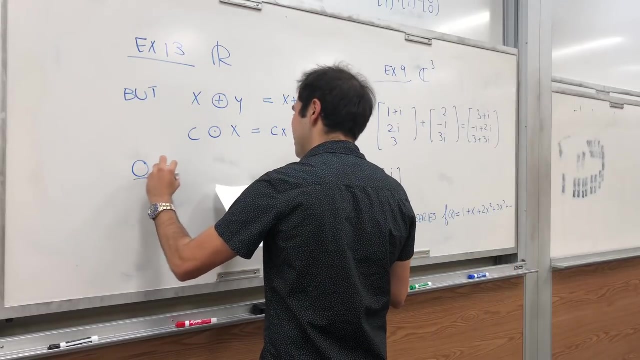 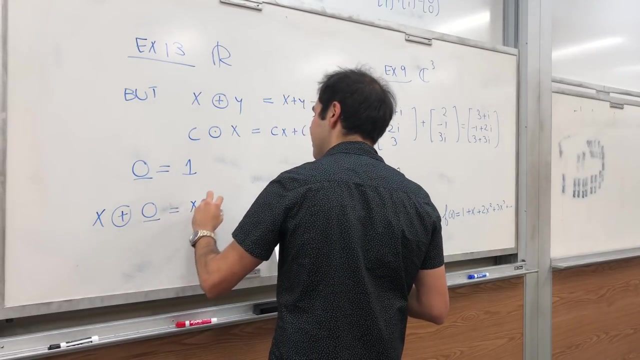 And multiplication c times x is cx plus 1 minus c. And what is really cool here? Here the number 1 becomes the new 0 vector, So 0 is just 1.. Why? Because take x plus the 0 vector, that's x plus 1,. 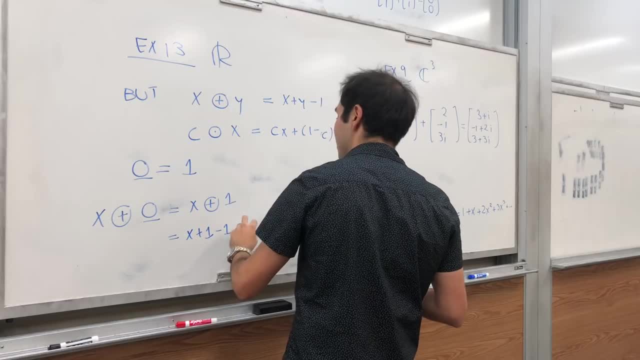 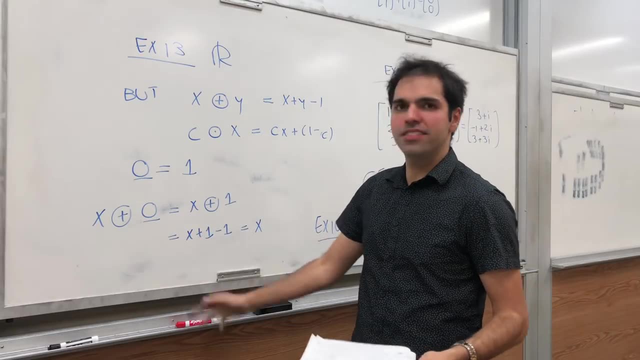 and that's x. plus 1 minus 1, and that's x. So you see, remember what the 0 vector does. It's a vector such that u plus 0 is 0, plus u, which is u, And that's fine. 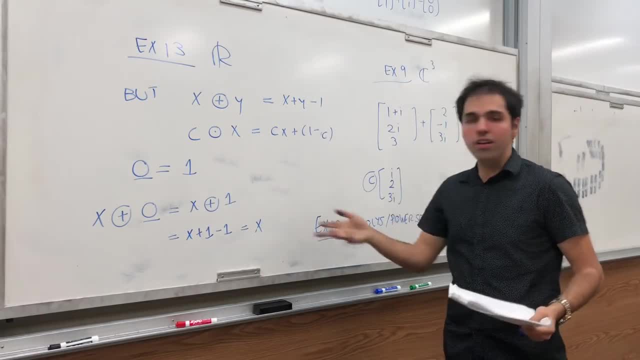 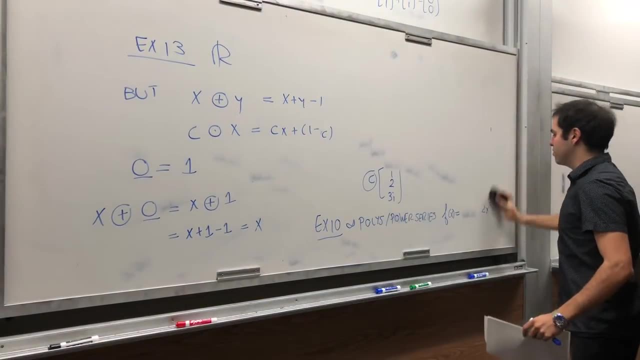 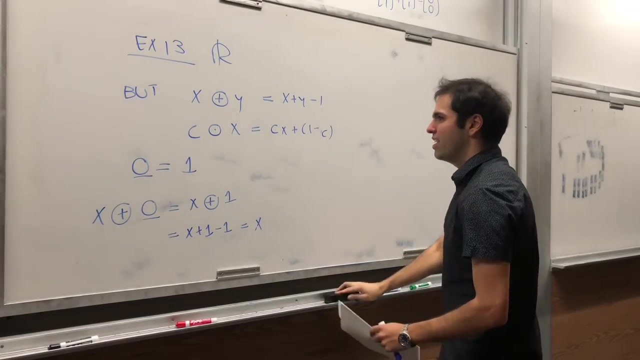 It's precisely what we've done. If you add x to the number 1, you just get x. It's kind of neat, I think 1, the number 1 is still the number 1 here. so that's fine, because 1 times x, yeah, is just 1.. 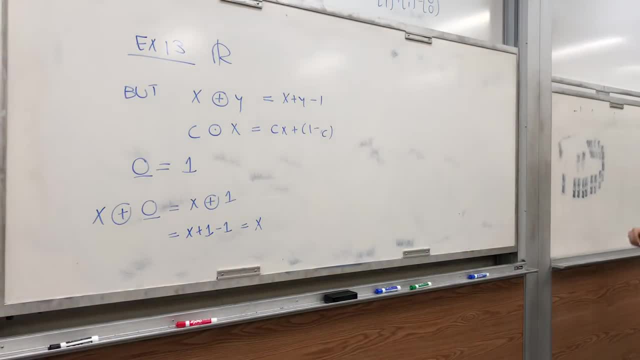 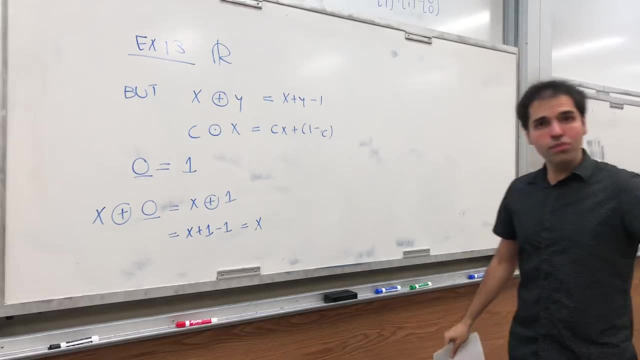 OK, so that was one example, And then I want to talk about other examples, sort of in a more general context. But turns out to want to show something as a vector space. you don't have to really check all those 10 examples. 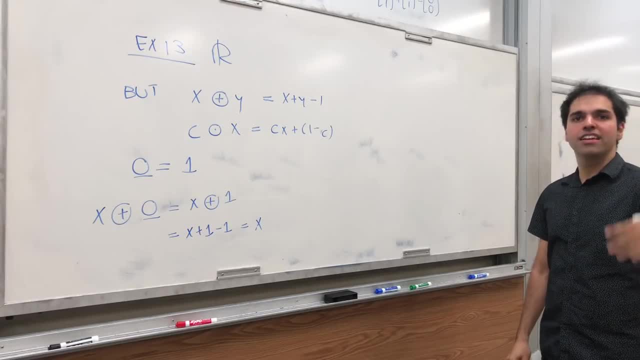 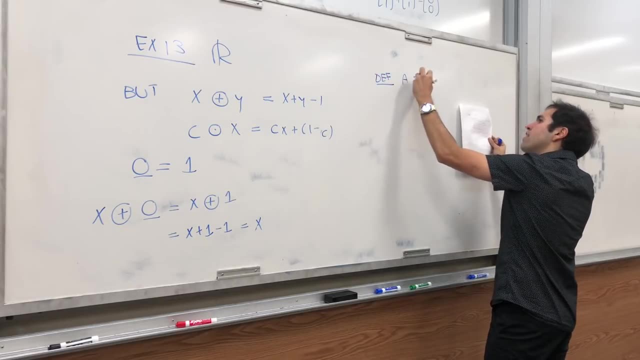 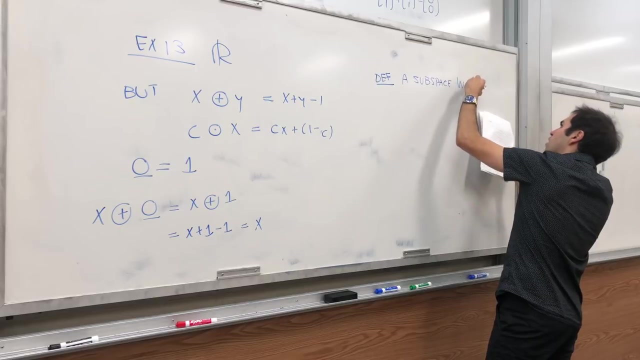 Because there's some cases where you can recognize something as a subspace of a vector space. So a subspace, so just a definition of subspace of v. so a subspace w of v, well, it's a subset of v such that 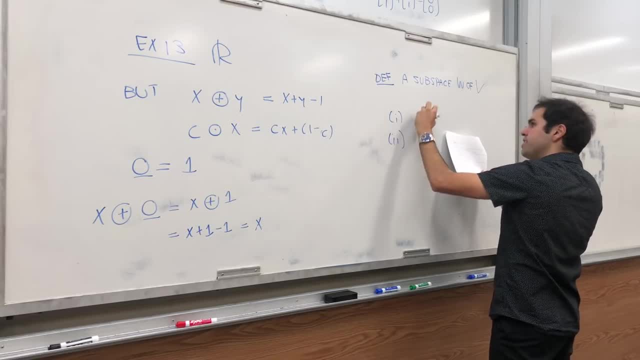 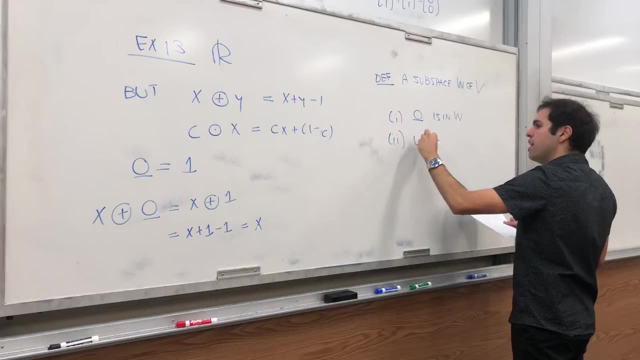 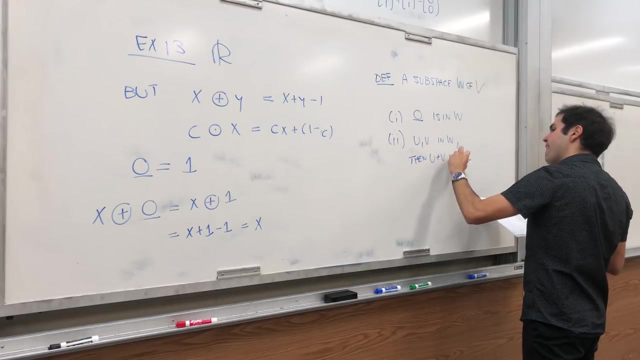 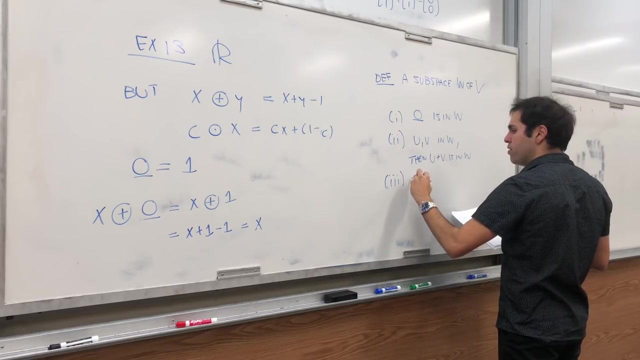 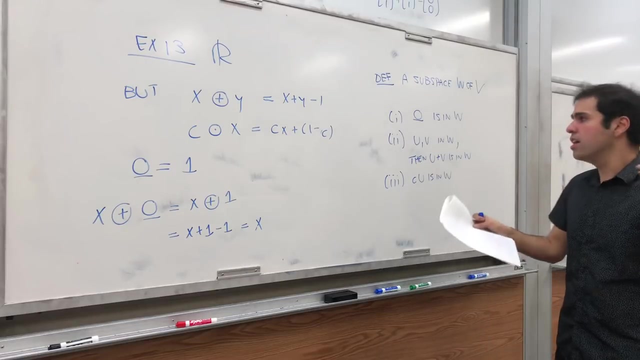 the following three whole: so the zero vector of V is in W and just the three properties. if you and V are in W, then u plus V is in W, and if you is in W and C is a number, then Cu is in W. so literally it's just a zero vector is in it. it's closed. 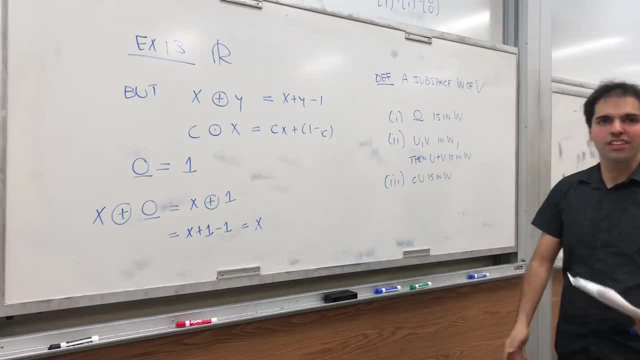 under addition and it's closed under scalar multiplication. in other words, if you're the set and you know it's a subset of a vector space, you only have to check those three properties because turns out, the other seven are then for free, and this thing allows us to find more things. so 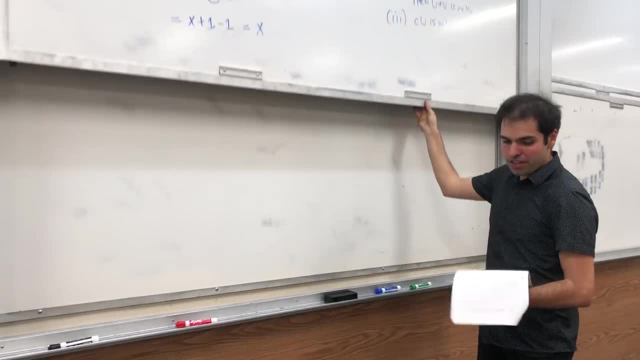 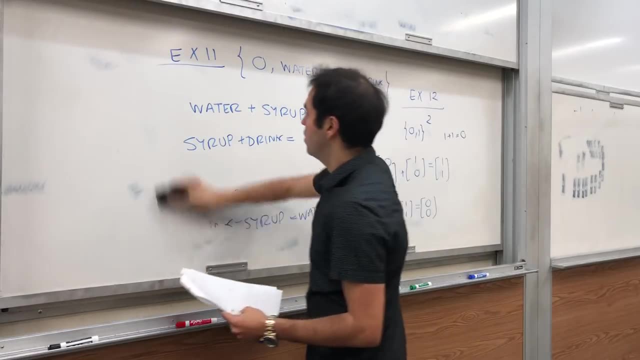 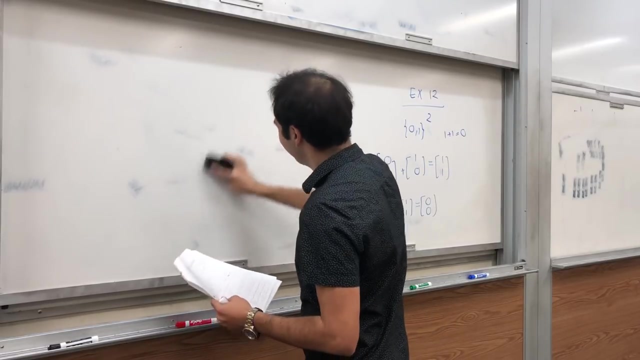 I'm going to show you how to do that in just a second. This allows us to generate more examples because, for example, you have a line through the origin and again, I'm not going to prove all those things because the end of the video would be one hour long, so that's not good. so example 14: a typical. 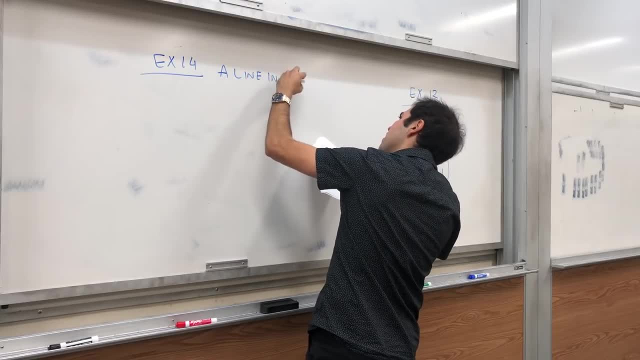 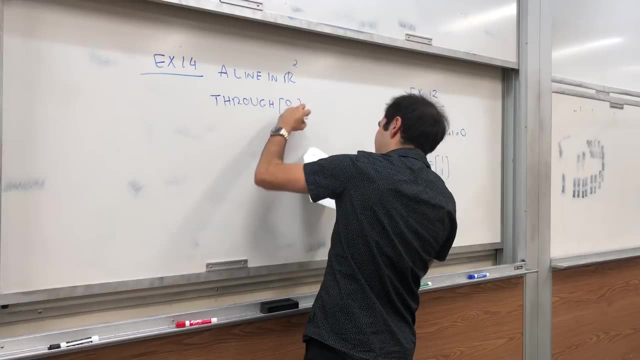 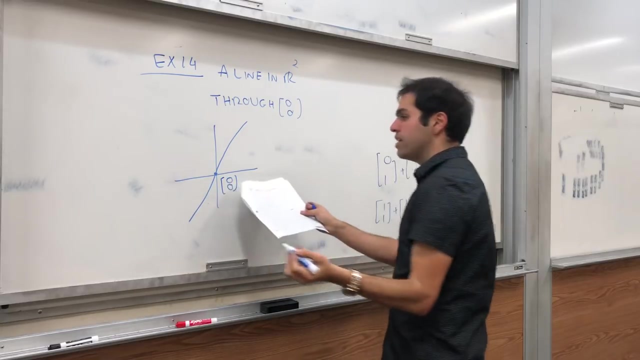 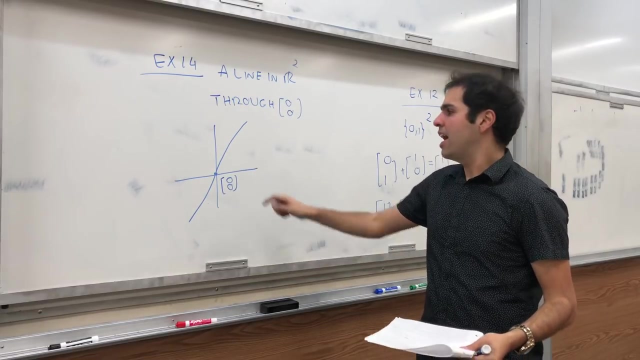 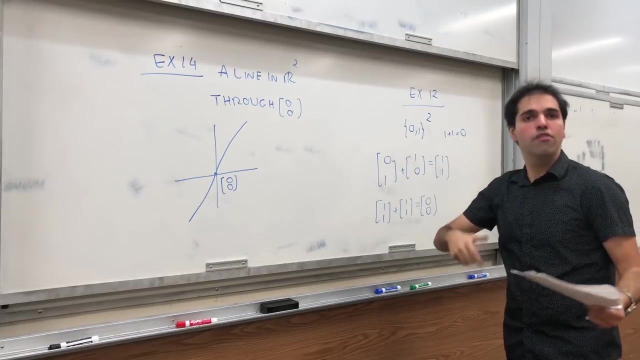 subspace is a line in R2, but the zero vector has to be in it, so it's through the origin. Okay, Okay, Okay, Okay, Something like that you have. this line goes through zero, zero. well, the zero vector is in it and you can show that if you add two vectors on this line, you still stay on this line, and if you scalar multiply a vector on this line, you're still on this line. so, indeed, it is a subspace of a known vector space, which is R2.. 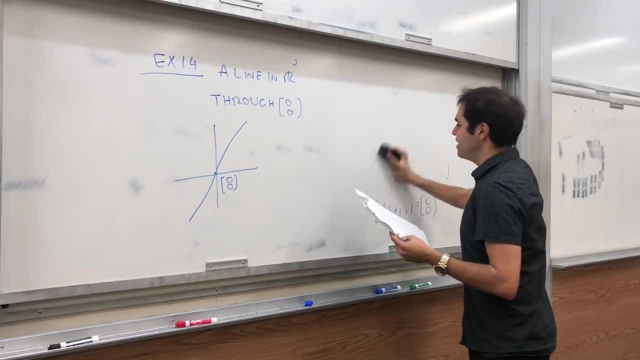 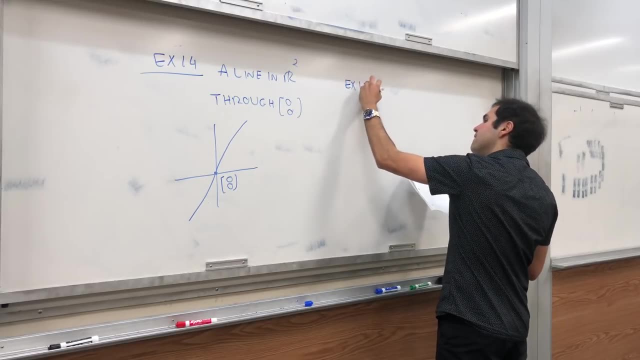 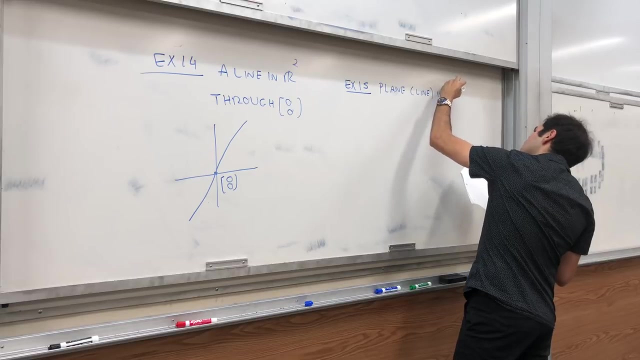 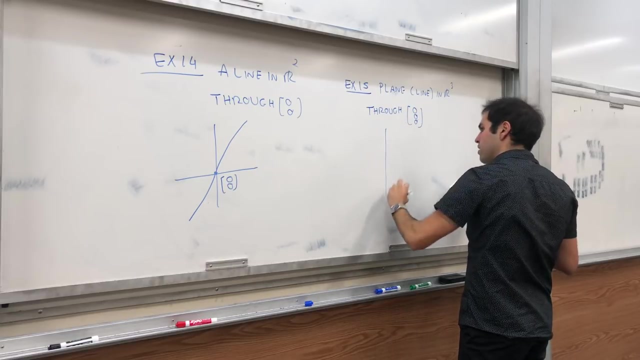 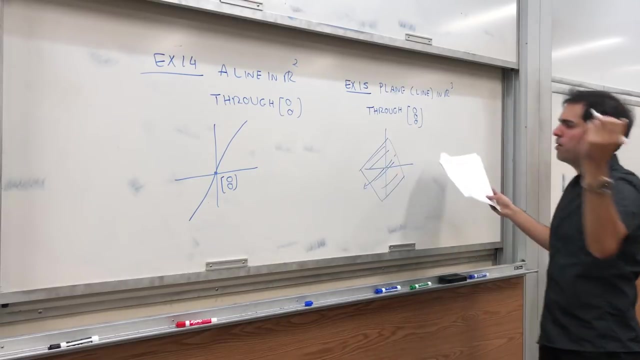 That was example 14.. Now example 15: similarly, a line or a plane in R3. so plane or line in R3 through this origin, zero, zero, zero. something like that you can also show it is a subspace of R3. so the point is, once you know the mother space, it's very easy to show something is a 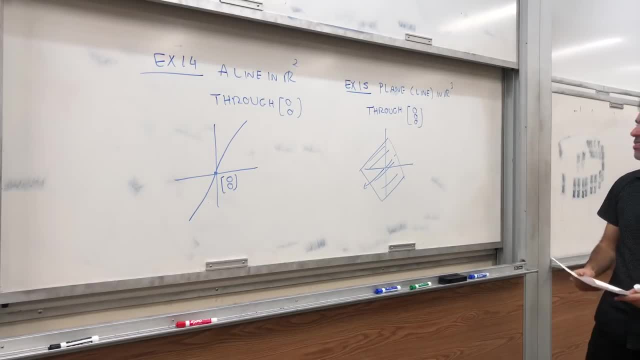 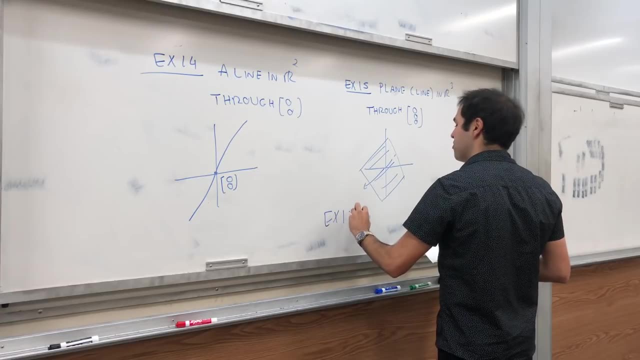 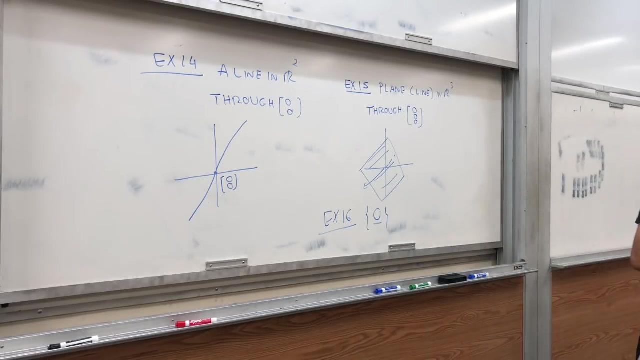 subspace. you just just show those three properties and in particular there is a very important subspace that's sort of trivial, so it's an oxymoron, but the zero space, so the space that just has a zero vector for any vector, space V, this is a 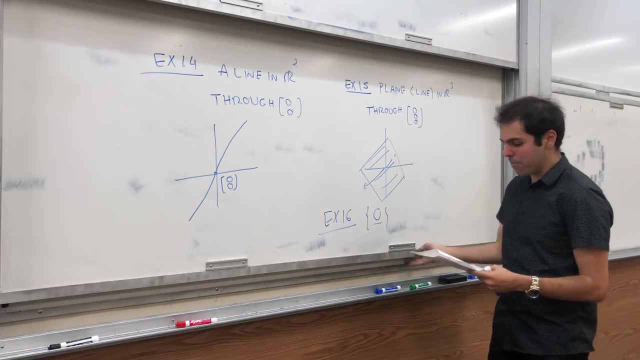 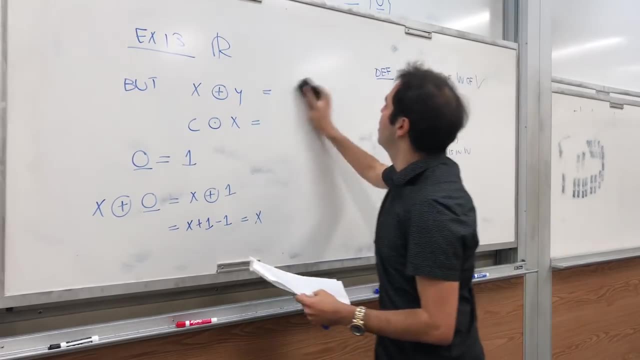 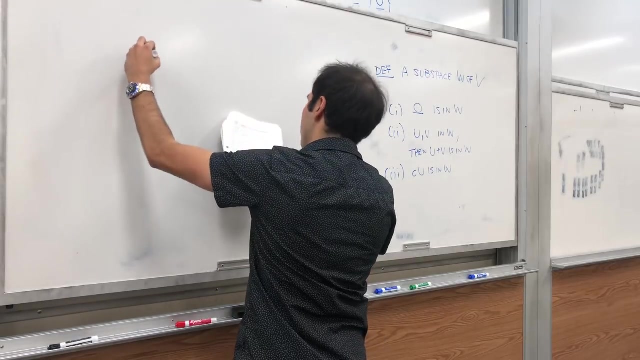 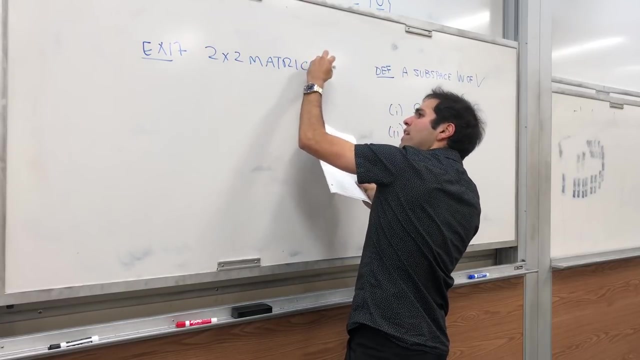 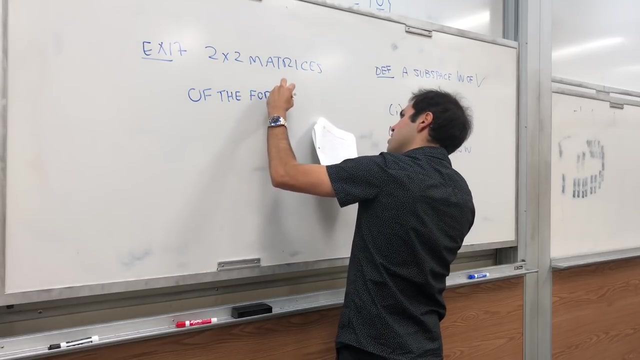 subspace of V. so which gives us yet another example. but then there are fancier ones that you can generate using this subspace technique. for example example 17: two by two matrices. so the mother vector space is a set of two by two matrices, but of the form a, b, zero, d. 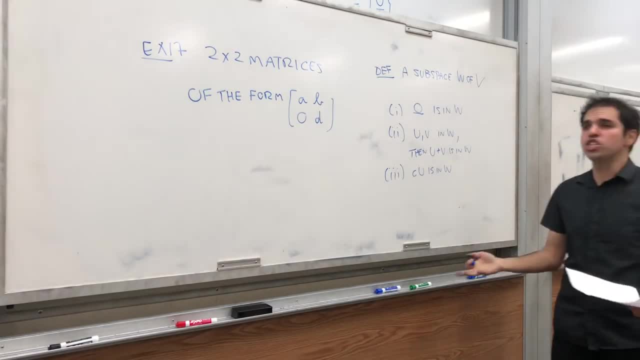 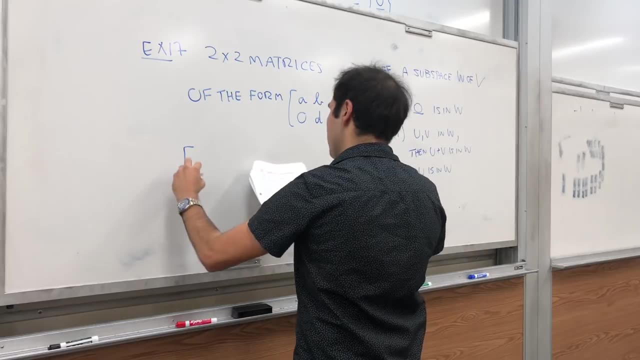 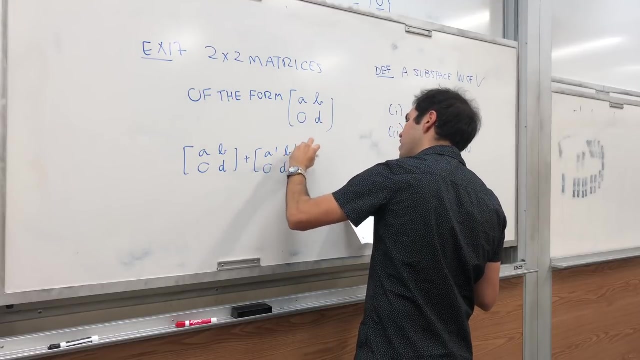 So, where this third entry is zero- and you can indeed check- if you take two matrices of this form and you add them, you get a matrix of this form, for example: you know: a b zero, d plus a prime, b prime, zero, D, prime, it is a plus a. 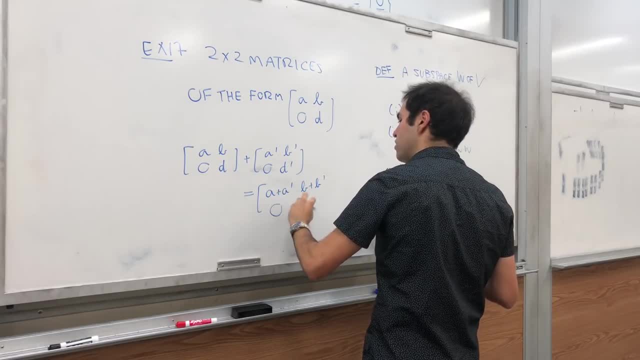 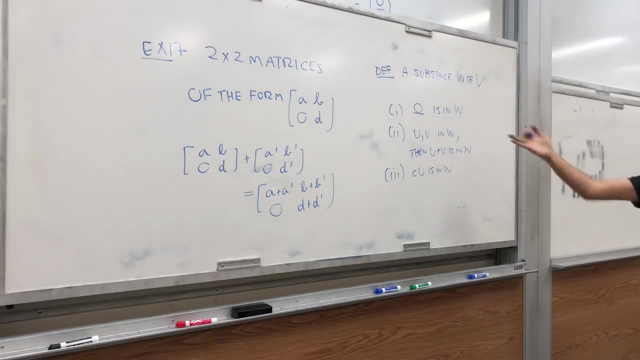 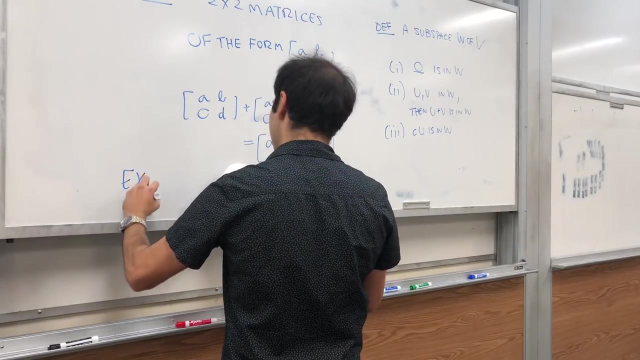 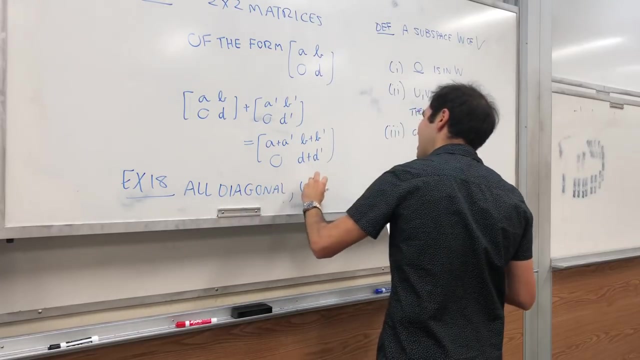 prime B plus B prime zero, D plus D prime, and indeed this last entry is zero, and So this gives us another example which is a subspace in this example. And of course, similarly, you have all diagonal, diagonal, or even upper triangular. 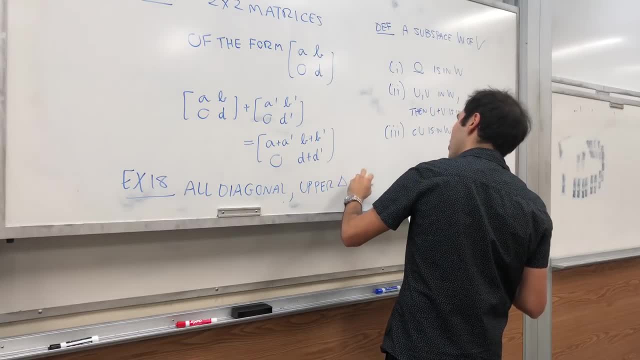 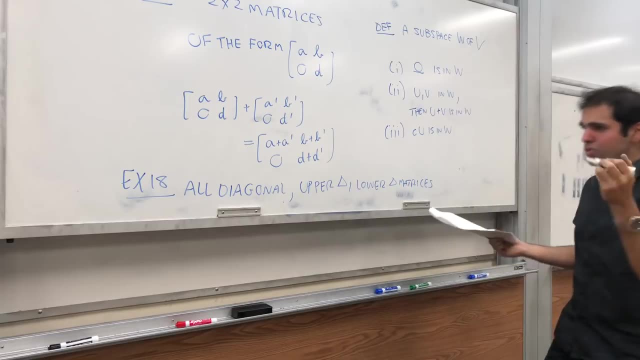 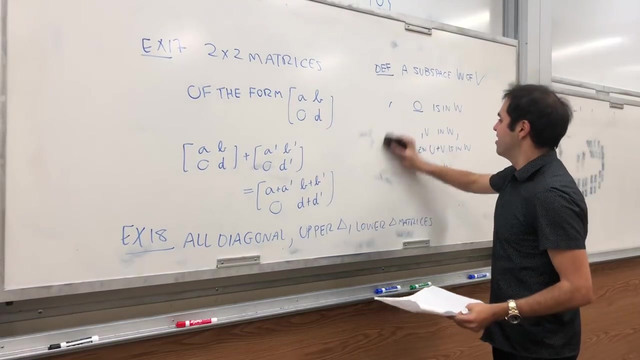 So this matrix is upper triangular or lower triangular matrices, So it's also an important subspace of the matrices, of, I guess in this case, 2 by 2, n by n matrices. So you see, there's so many of them and they're all so useful. 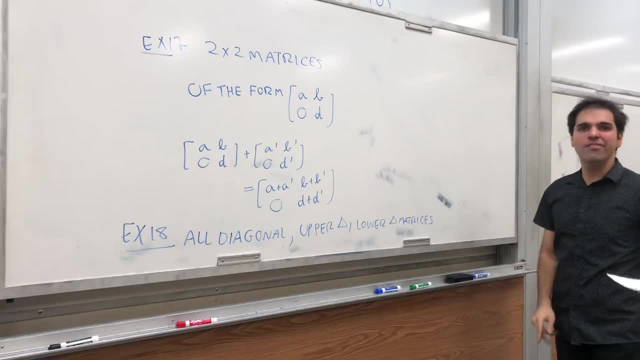 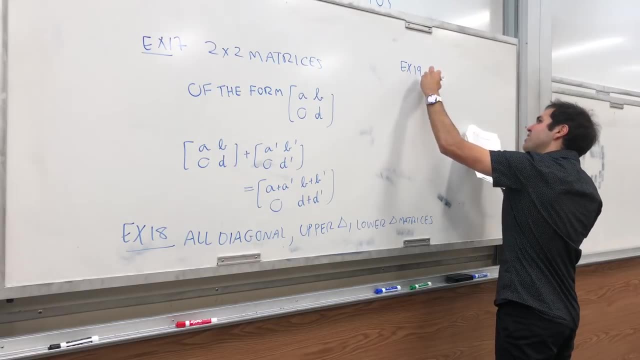 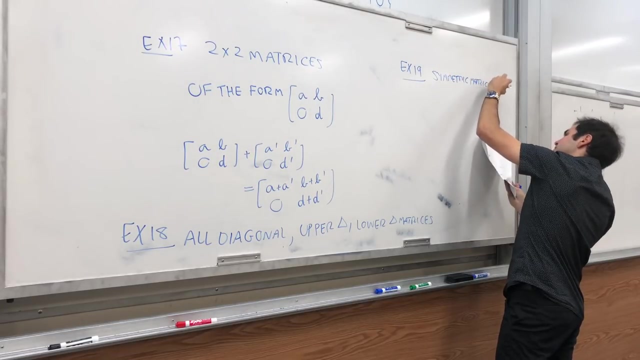 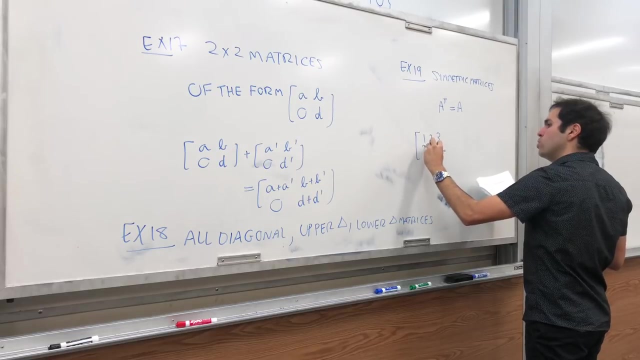 See, that's why we're not wasting your time by teaching you about vector spaces, because all our theory applies to all those examples. Okay, another one: symmetric matrices, Matrices where A transpose equals A. So you know, for example, 1, 2,, 3,, 2,, 4, 5, and then 3,, 5,, 6.. 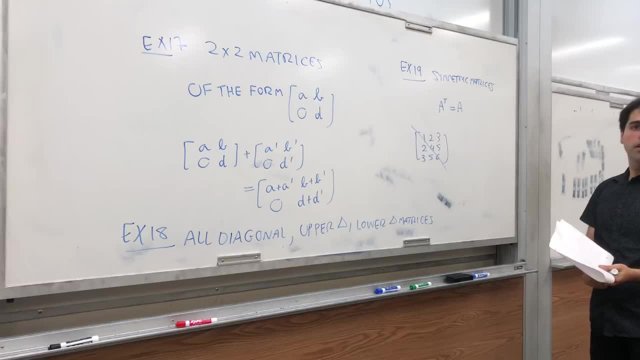 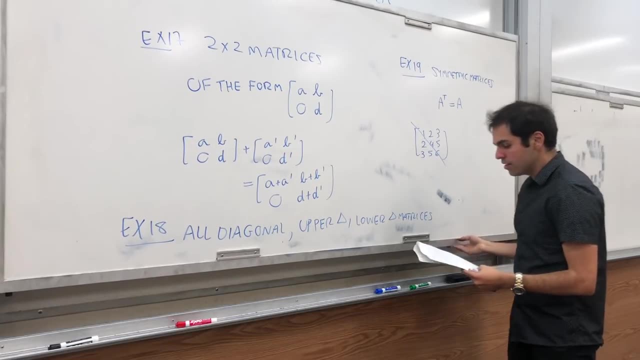 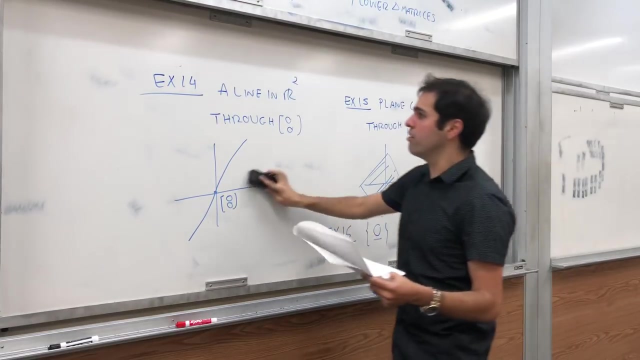 It's a matrix that's symmetric along the main diagonal. This thing, the set of those matrices, also forms a subspace, hence a vector space. And, going back to our functions, You can generate other kinds of vector spaces, So more specific polynomials. 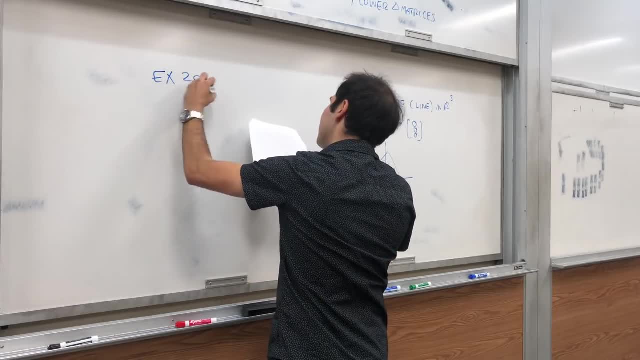 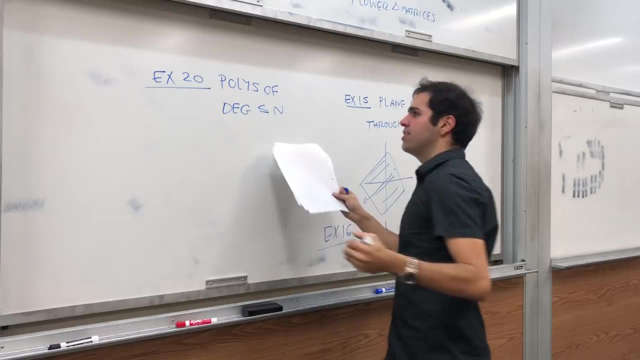 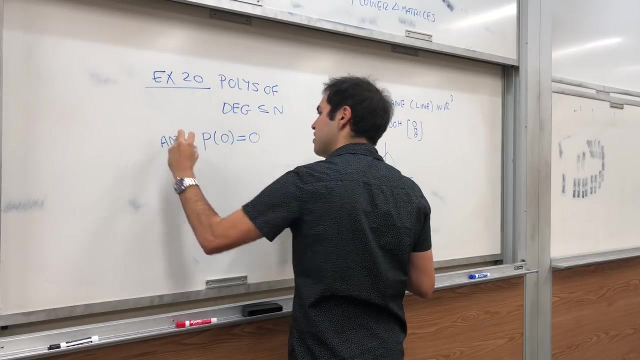 So, oh, already at 20,. okay, example 20.. Polynomials of degree less than or equal to n. So that's our mother space, but with the requirement that p of 0 is 0. So, think you know x squared? well, I don't know. x squared plus 3x. 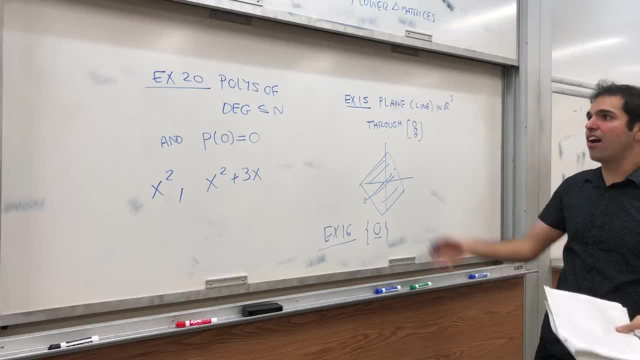 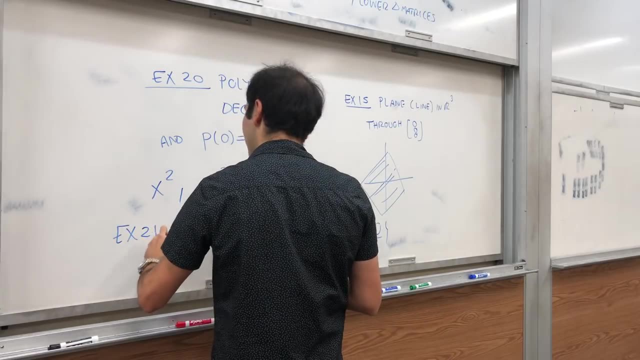 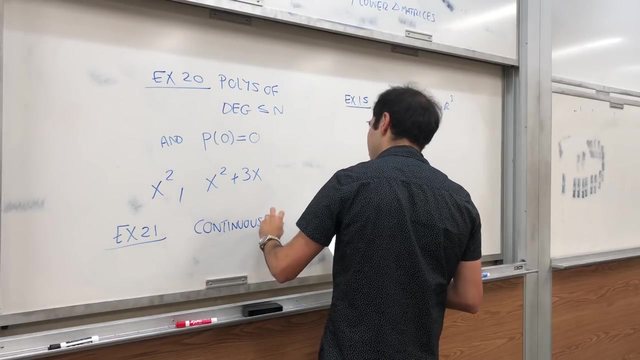 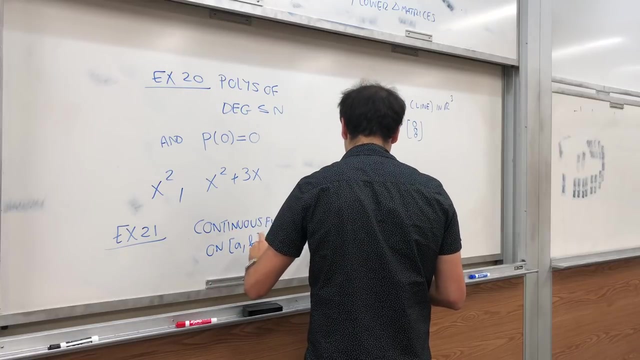 You see, basically polynomials without constant terms. Those also form a subspace, hence a vector space, And one thing I alluded to is basically the set of continuous functions. There's a super important vector space in applications. So, on an interval, AB, so CAB and you can generalize this. 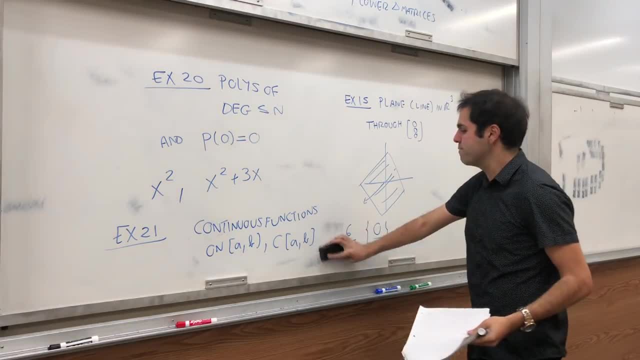 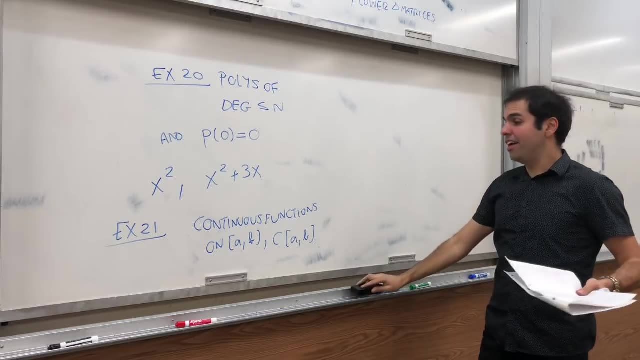 I think, all integrable functions. in whichever sense you like, they're also a vector space, Because they're just a subspace of the set of all functions. And in particular, it is true, if you add two continuous functions, you get a continuous function. 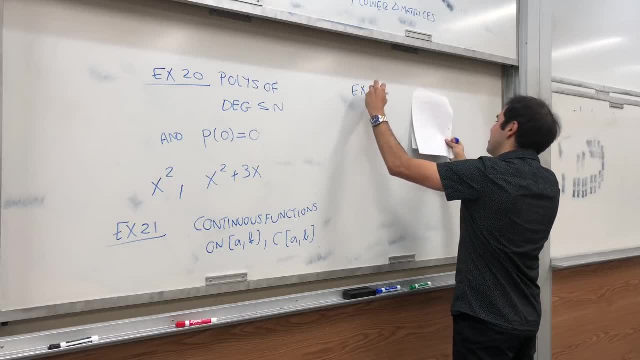 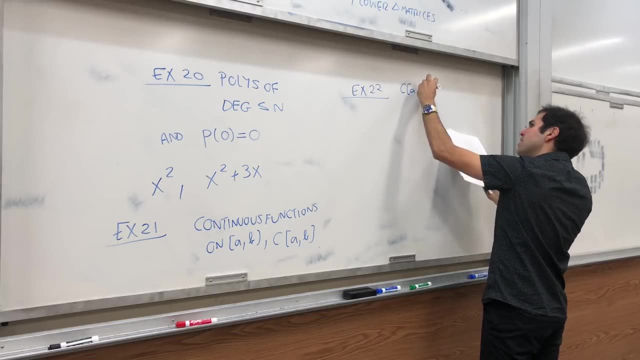 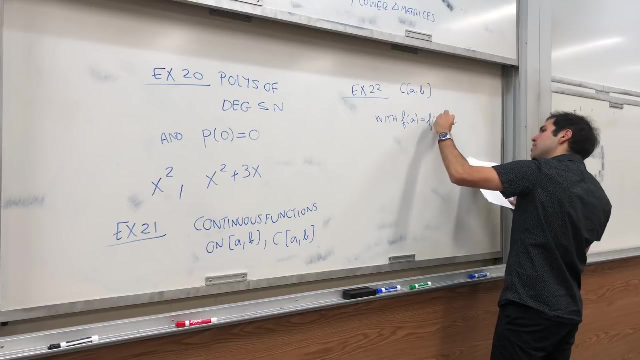 And similarly you can scale or multiply a continuous function and get a continuous function. And also, for example, the set of CAB, again set of continuous functions with a set of continuous functions, If f of A equals to f of B, so basically functions whose initial value is equal. 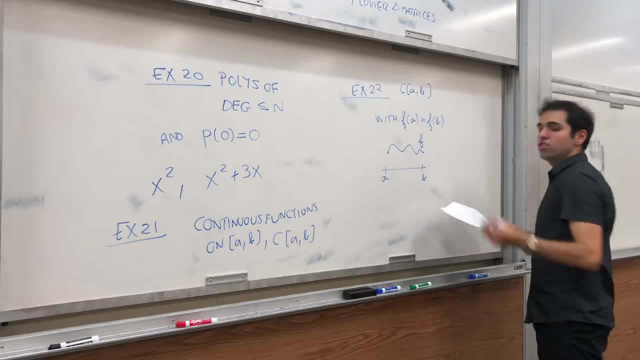 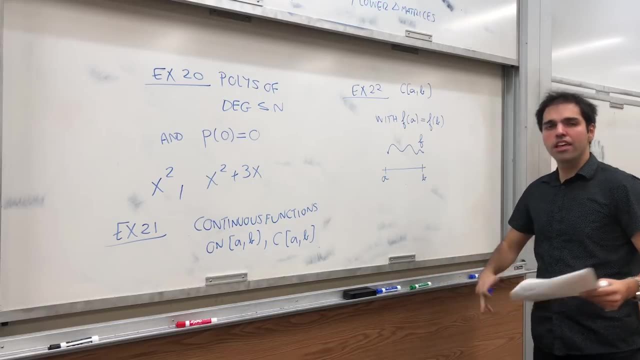 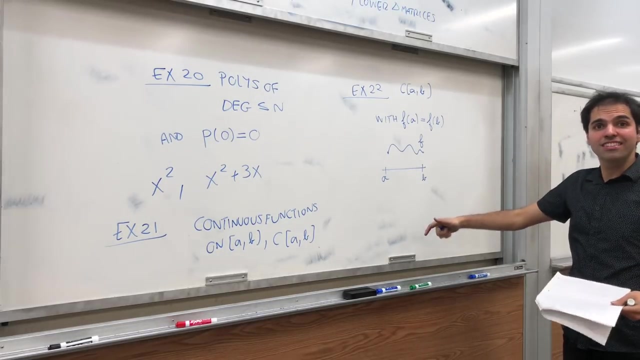 to its final value. also check that If you add two functions with the same initial value, so whose initial value is this final value? then for f plus g, the initial value will be the final value. In particular, periodic functions of a fixed period. 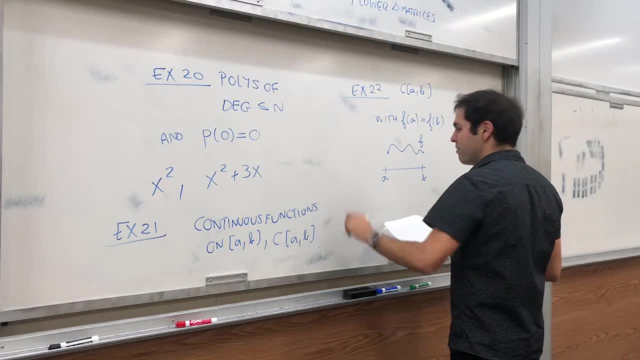 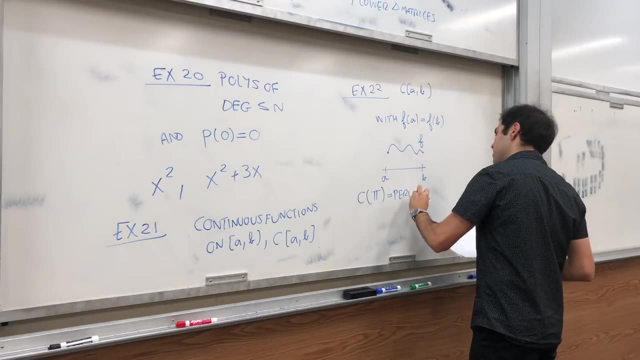 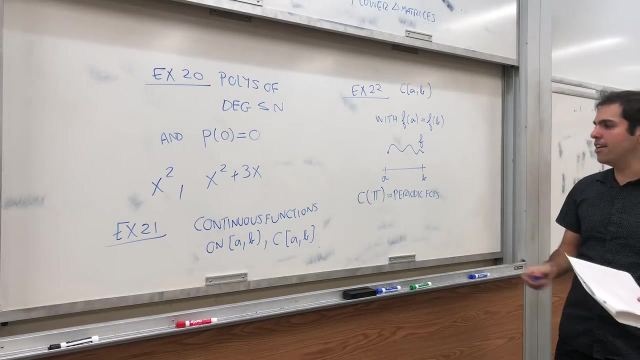 that also forms a vector space, sometimes called continuous functions on the torus, so CT, so periodic function. It's interesting to find a basis for CT. Basically that's how, like Fourier, analysis, is generated. right, Because a basis would be just the exponential functions. you know, EI something. 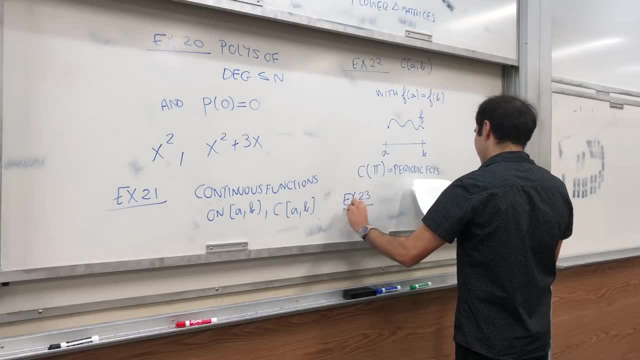 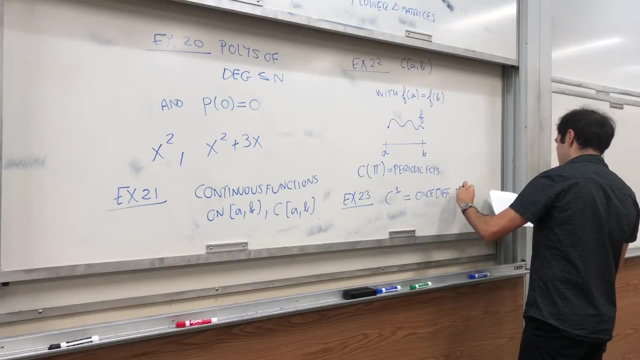 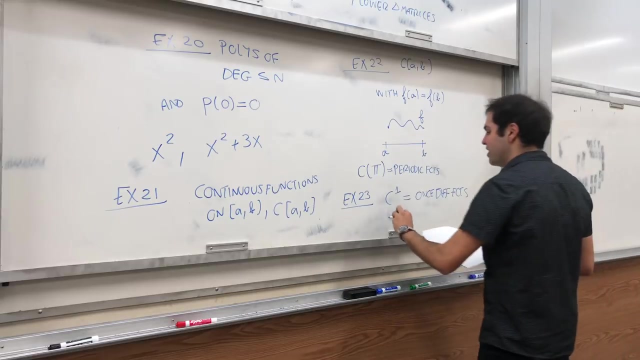 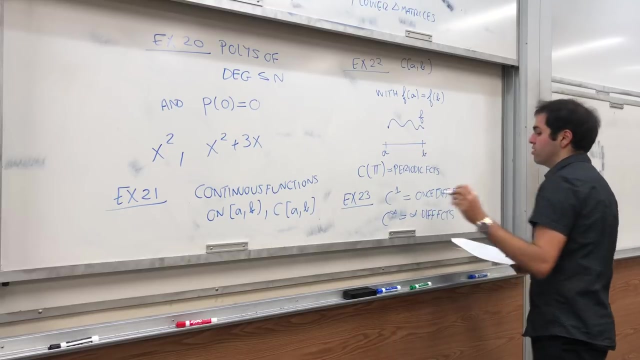 And, of course, similar to that. you can have a difference like C1,, which is once differentiable functions whose derivative is continuous. There's a very important space in geometry, or C infinity: infinitely differentiable functions, Differential equations. that's so important. 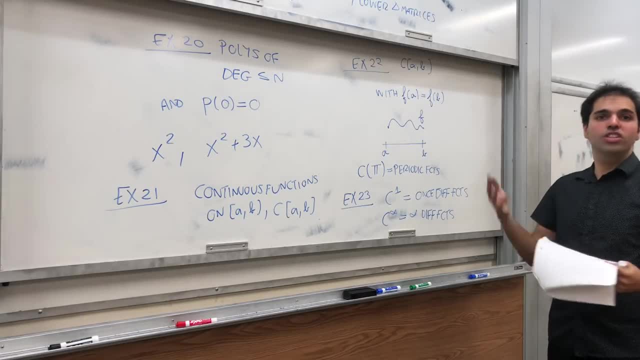 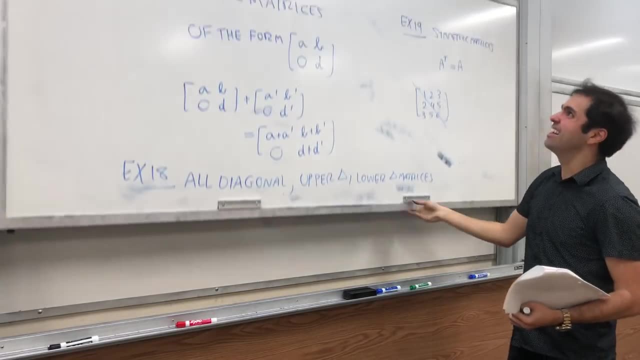 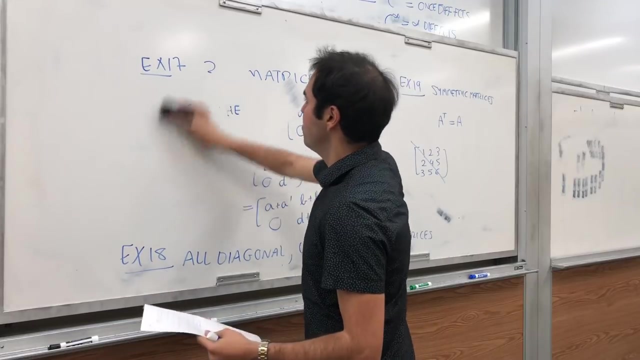 Or something called analytic functions, again functions which have power series, Also super important and complex, Complex analysis, for example. and ah, we're almost done. So 23 examples, two more to go, So another one. it's simply so. there are some other very important spaces. 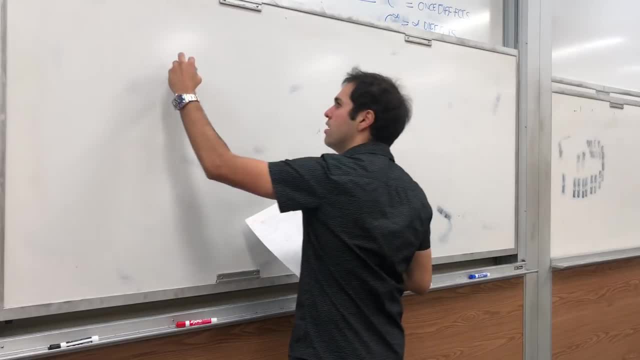 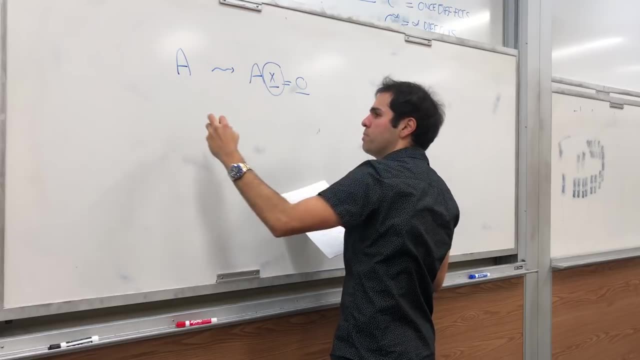 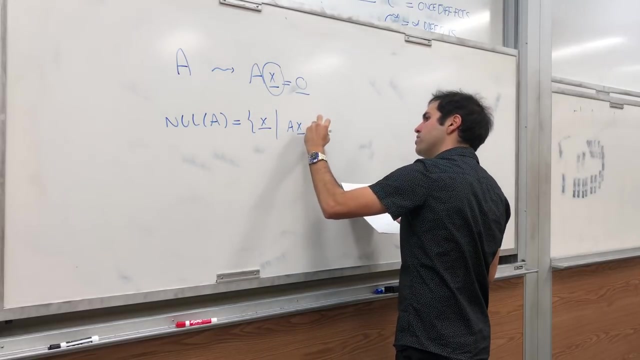 So, basically, if you have a matrix A and you look at the set of solutions of AX equals 0, right, That is what's called a null space. So null of A is just the set of X where AX equals 0.. 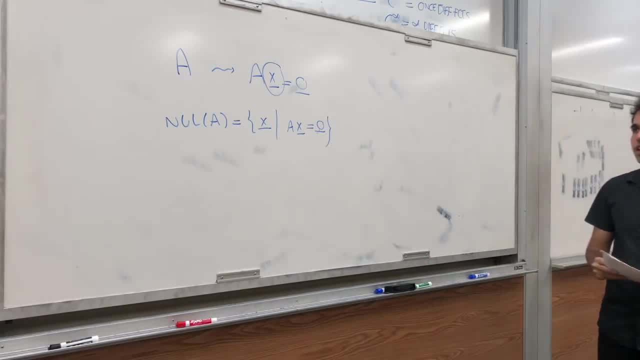 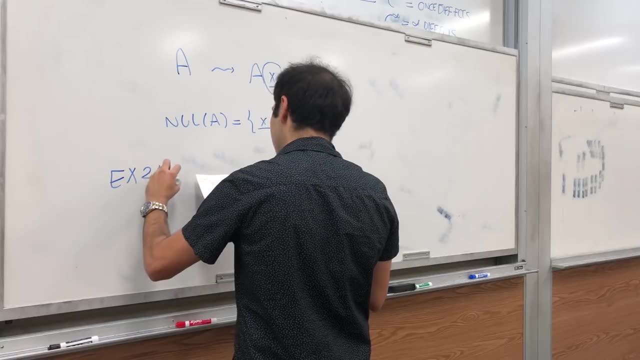 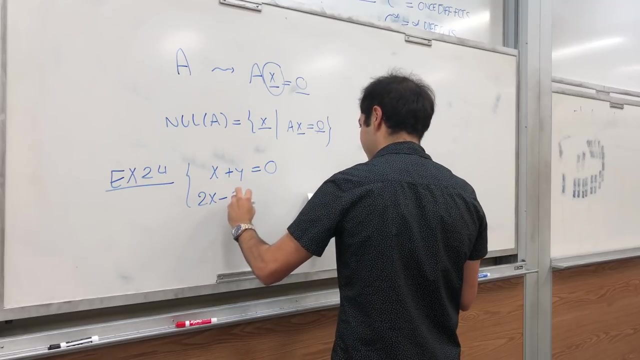 And it turns out- and I've shown this in another video- null of A is always a subspace. So, for example, if you take the set of solutions of X plus Y equals 0, and 2X minus Z equals 0,. 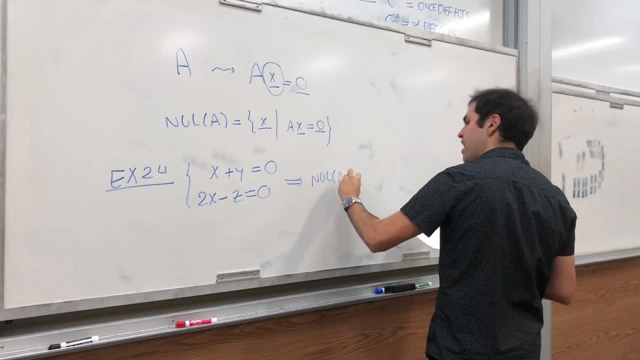 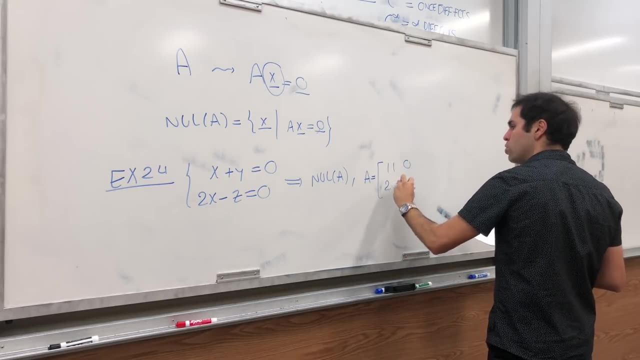 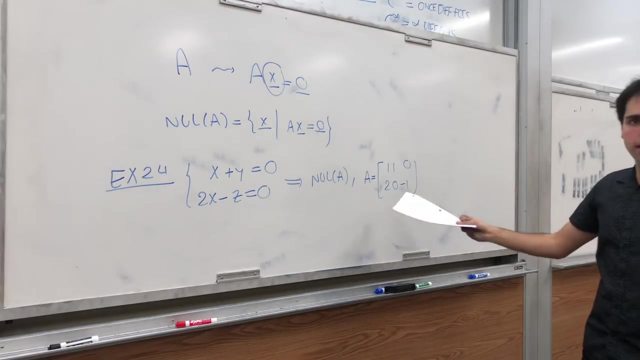 well, you can write this as null space of A, where A equals goes to a matrix, I think 1, 1, 0, 2, 0, minus 1.. And by what I've shown, this is automatically a subspace and therefore a vector space. 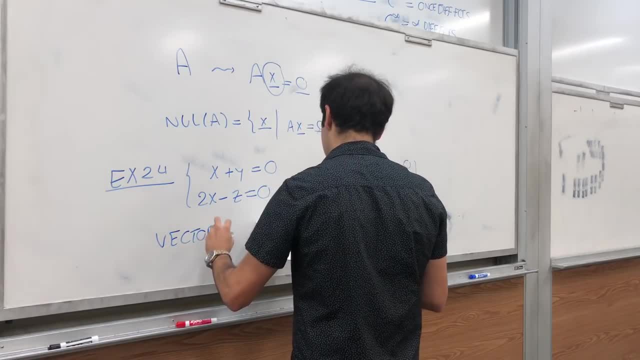 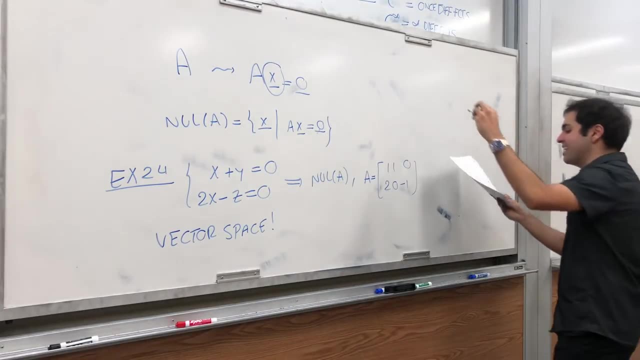 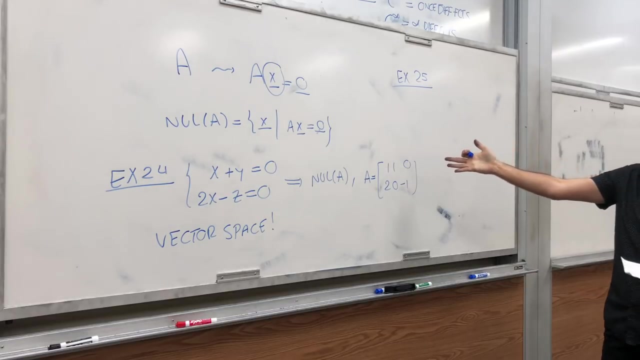 So this is also a vector space. Of course you can write this as a line, but still it's kind of cool Just abstracting. And not only does this work. so I guess this is one of my final examples- not only does this work for matrices.